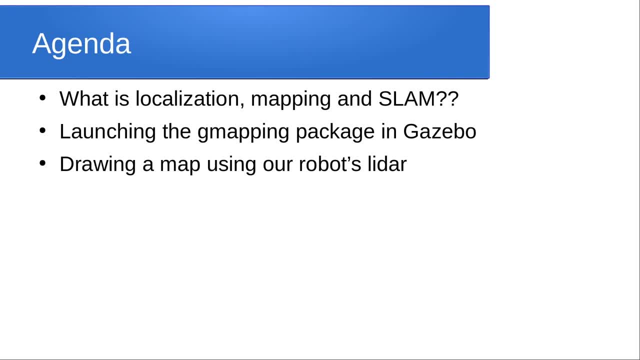 So today we're going to define something called localization, also mapping and SLAM, And we're going to get introduced to each one of these terms and we're going to have some basic definitions and like the simplest form of explanation for these three terms. 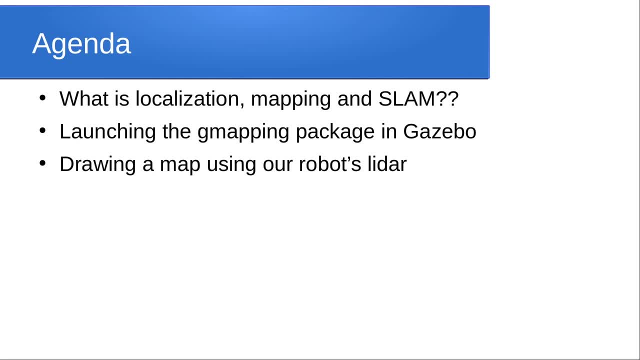 And we're going to launch the gmapping package in Gazebo and that is a SLAM package, right, And then we're going to draw a map using a robot slider. So we're going to draw a map for the environment or for the world we're located in. 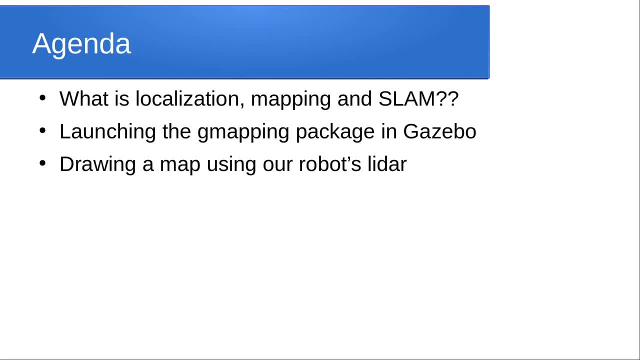 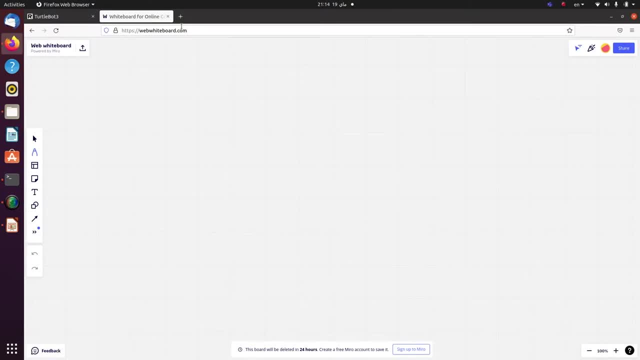 And we're going to define what a LIDAR is. So let's dive in. So, before getting our hands dirty, we need to get introduced to some theoretical terms that will be quite useful for us and are quite important to understand and comprehend. So, first of all, we have something called localization, and for that we'll assume that our robot is. 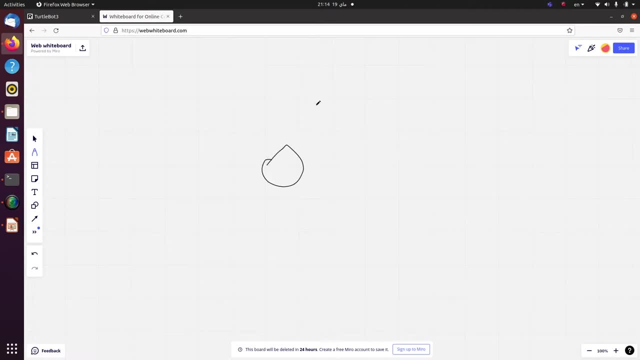 here. So it's located somewhere here in my world and let's just assume that the global reference frame of my world is here. So we've got, like, our x-axis, our y-axis and we've got the z-axis pointing out of the page. 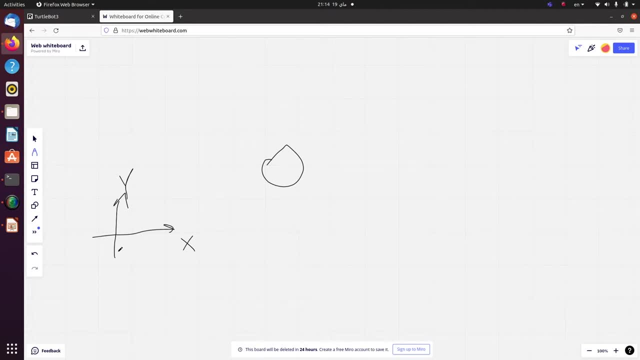 So we always assume that the height of our robot is zero, since our robot is located, you know, on ground level, Or it may be just like, translated a little bit, in the z-direction, depending on where the center of our robot model is. But anyway, we can assume that the z-distance or the z-coordinate of our robot is always. 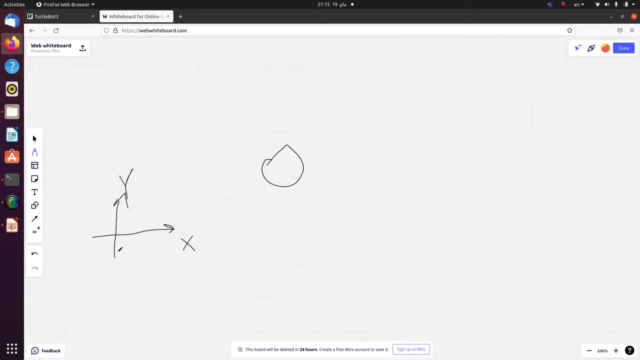 zero when it comes to wheeled mobile robots. Of course, that's not the case for other mobile robots, like drones, for example, or quadrotors, which have, like, variable height depending on the thrust of its thrusters. The same thing goes for autonomous underwater vehicles or remotely operated underwater vehicles. which have six degrees of freedom underwater. So we can assume that the z-distance or the z-coordinate of our robot is always zero when it comes to wheeled mobile robots. So we can assume that the z-distance or the z-coordinate of our robot is always zero when 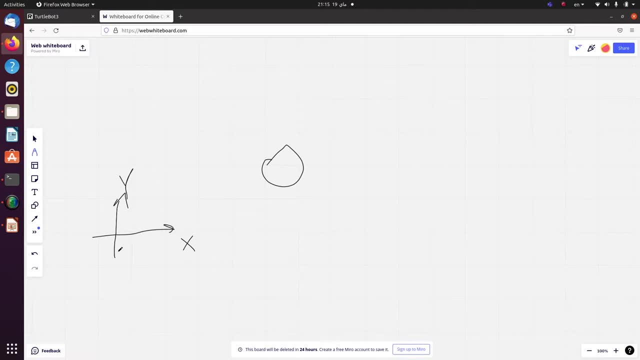 it comes to wheeled mobile robots. So we can assume that the z-distance or the z-coordinate of our robot is always zero when it comes to wheeled mobile robots- And there are also many types of robots- We've got humanoid robots, for example, and actually their center is always oscillating. 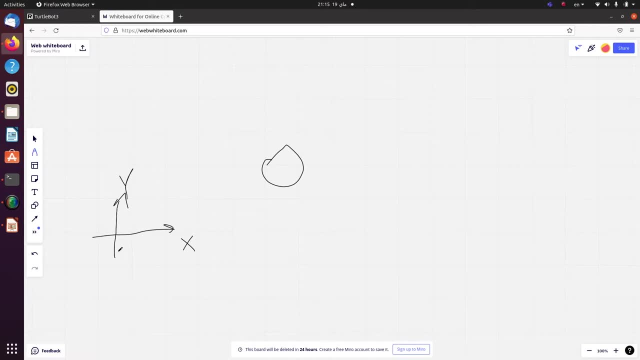 like in a sine wave fashion, because the center of mass like follows a sine trajectory or an almost sine trajectory during walking. So we'll assume we have a wheeled mobile robot here. so our z-coordinate is always constant, but our x and y-coordinates are, you know, very similar. 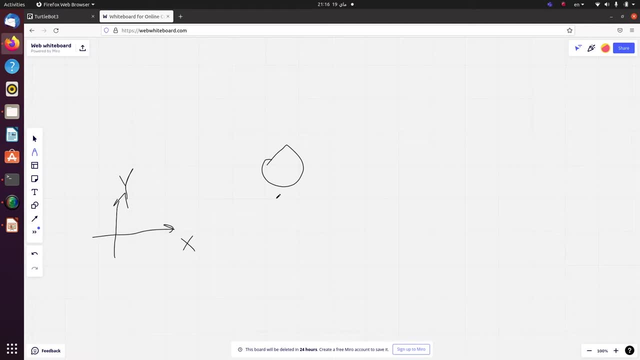 variable and the change during the simulation. So one of my tasks as a ROS developer is to develop some module called localization module. So the word localization means is to determine my global pose relative to the global frame. So I need to determine my global x, I need to. 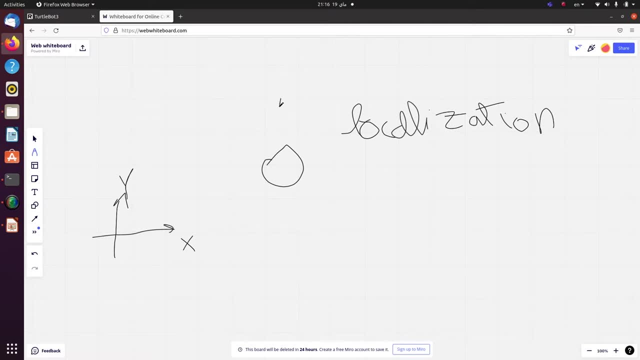 determine my global y and, of course, I need to determine my theta, which is the yaw angle. The roll and pitch angles are always assumed to be zero because we have like some restriction forces which are the ground reaction forces, because we have like two actuation wheels. 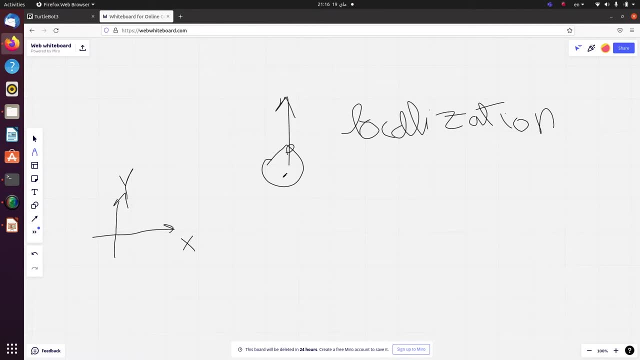 and two custer wheels. and what a custer wheel is? it's like a support wheel here. So all those have, like the main wheels, the right and left wheels, which are the main wheels, and the right and left wheels, which are the custer wheels. 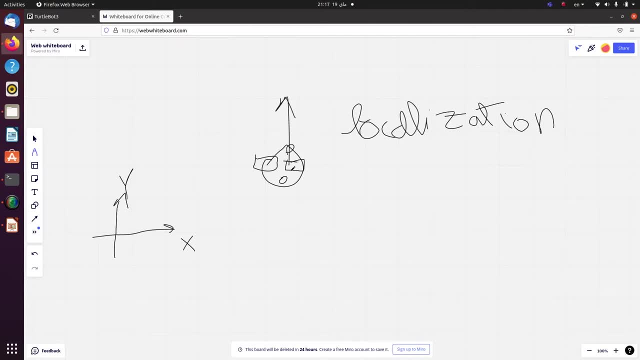 are responsible for actuation motion, and two custer wheels, which look like, you know, your stroller wheels, or like supermarket cart wheels, which you know, which do not help actuate your vehicle. They're just there in order to provide support and they have, like you know, multiple degrees of freedom so they don't restrict. 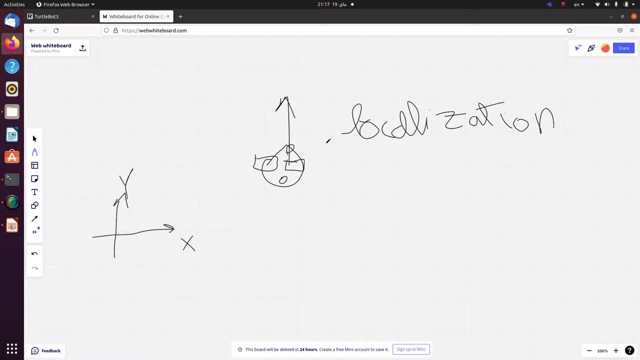 any motion. They're just here to support the vehicle, so that the vehicle does not tilt forward or backwards, So we can assume that the roll pitch angles are always zero, Right. so this is what's meant by localization, and in order to localize our robot here, we need to have 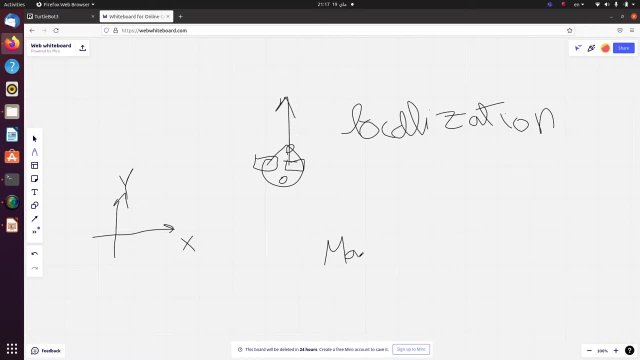 a map. So we need to have a predetermined map for this environment, and by map I mean like we need to have some 2D map describing the location of walls, for example, and describing the location of objects, Like this, for example. right, So our map basically is going to be, you know, like a whiteboard, with 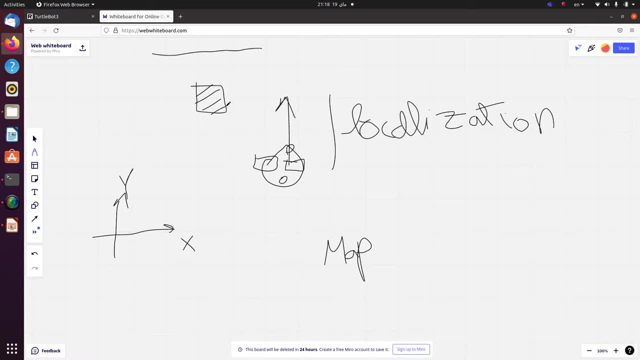 some black lines or black areas, where these black areas determine the position of obstacles or the coordinates of obstacles that the robot is not supposed to, you know, go through or collide with. And by knowing our map we can localize the robot, How. The robot has some sensor here called the lidar. 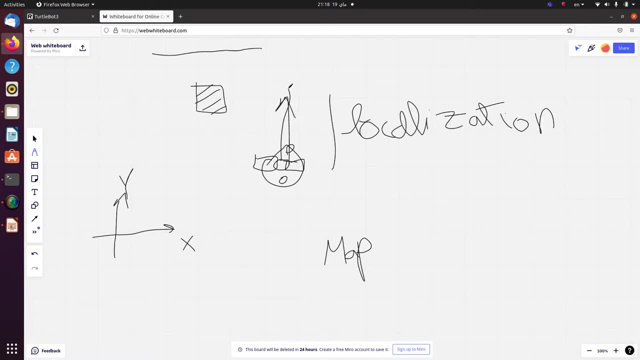 So what the lidar does is that it produces like laser beams, all right, and once these laser beams hit some object here, the laser beam retracts here and gets back to the lidar and the lidar computes the distance to that object through the computation of the time of flight. It's basically. 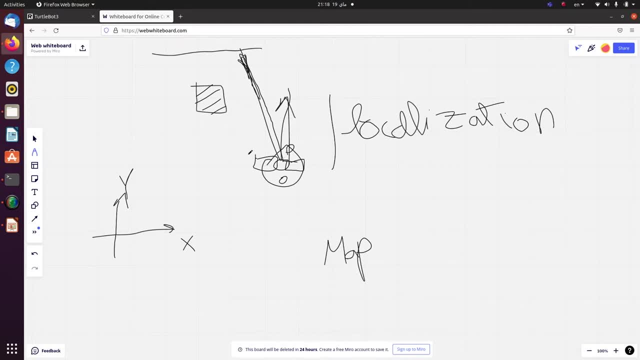 like sonar, And the lidar is rotating. so we we've got a family of lidars called 360 lidars, which produce several beams in all directions, in all the 360 directions or 360 degrees. Sometimes lidars, just you know like send beams in a span of 180 degrees. instead, 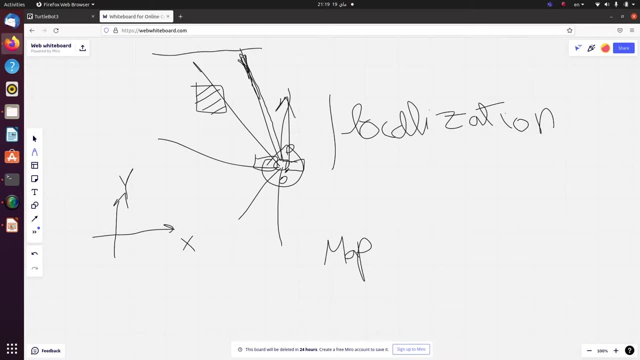 of full 360 degrees. But let's just assume that we have a lidar that produces beams and keeps rotating. It's like shooting laser beams and rotating at the same time. so we get like a local map which determines, you know, the current observations in my environment, the current 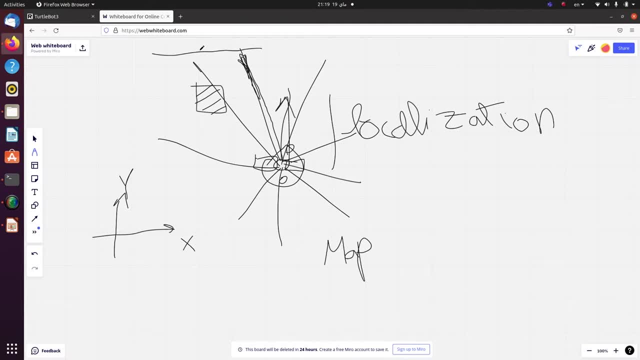 depth of objects that I've located so far, And this laser beam has a range, and what I mean by range is the maximum length of this laser beam, after which I'm not able to compute the distance to the object. maybe the object is too far and I cannot locate it, so whenever I'm walking I'm just taking, like. 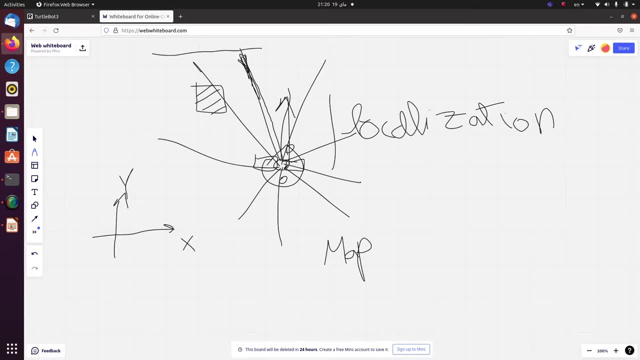 2d images of my current environment and I'm trying to determine the black dots or the obstacles in this environment while I'm walking or while I'm moving right. so by knowing this map, we can determine the location of the robot. and, for example, let's just say: 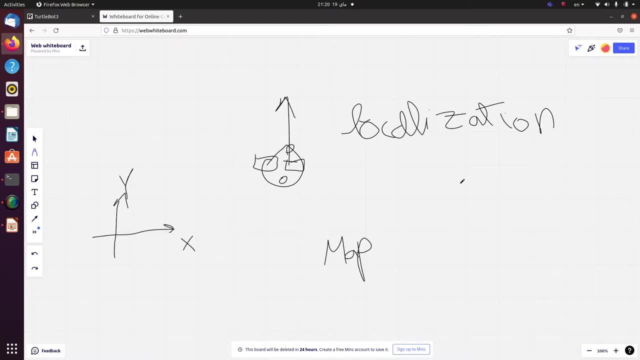 let's just say the robot was here somewhere right in my environment. so my first observation was that I found like a wall here right thanks to my rotating lidar, and during one span of the lidar I just detected these walls, for example right. so when I moved a little bit and 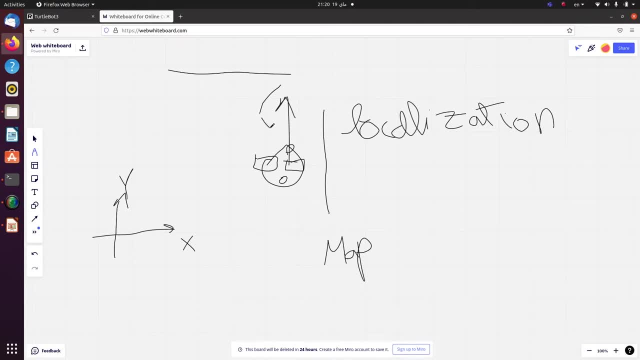 the robot changed its position to be here, for example. so the robot was basically moving forward and the robot became here. I take another set of observations and this time my observations reveal that the walls are getting. this wall, for example, here, got closer to me, because this is a relative 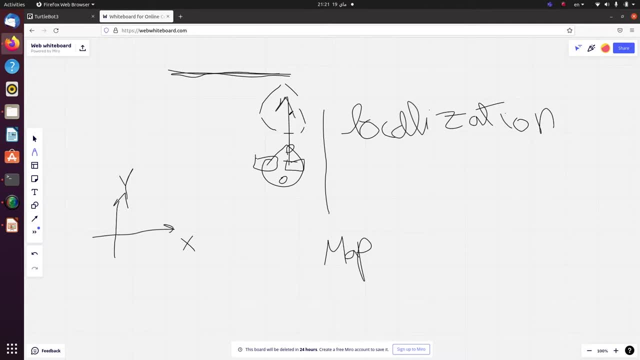 measurement: you getting closer to the wall is equivalent to the wall getting close to you while you're static. it's like the train observation effect. all right, so we found that the new readings. well, this is the new readings, and this is the new readings, and this is the new readings. 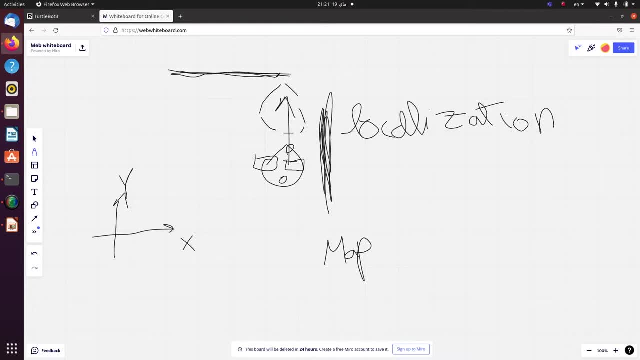 this wall didn't move and this wall is like getting closer to me and I can deduce through this observation or by comparing the two observations, the past observation and the current observation, that the robot has moved like a distance for, for example, if this wall got closer. 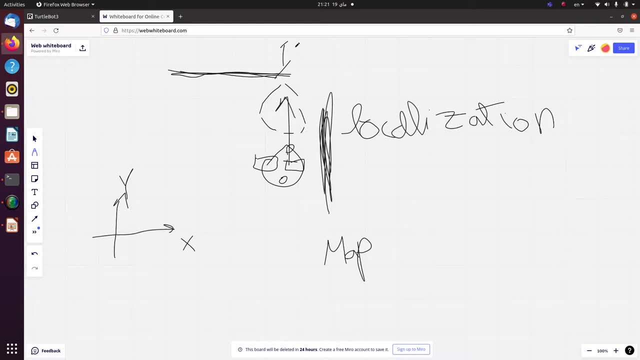 by, for example, one meter, then that actually means that the robot has moved forward for a one meter, and this is a pretty simple explanation of what's going on. it's actually a bit, you know, more complex than that, but this is a simple example to let you, you know, have the intuition of what's. 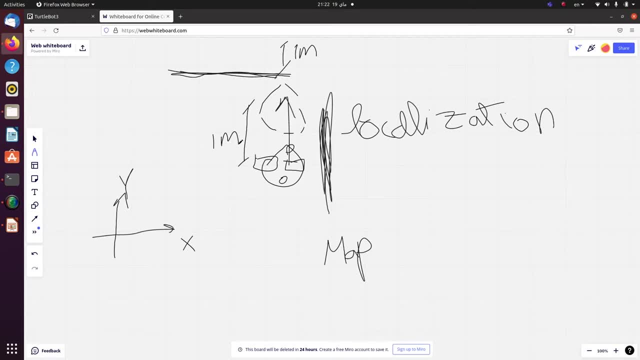 going on. so this is how localization works, right. there are other sensors that you know are subsets of this localization process as well. you might have an IMU, all right, which computes the acceleration and the IMU. through this computation of acceleration, you can double integrate this acceleration value in order to get an estimation of how much he moved. so, for example, your IMU is: 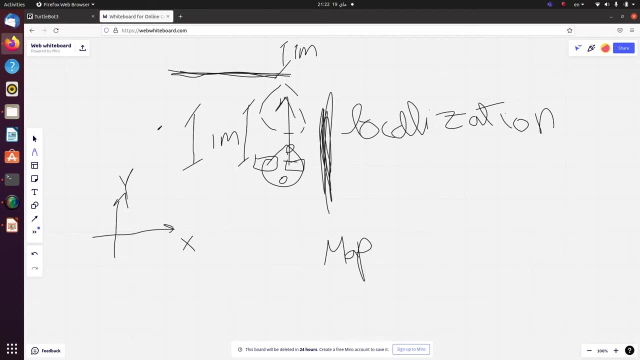 noisy, so it will give you a reading that basically says that the robot moved, for example, 1.2 meters instead of one meter because, as we said before, any process that includes integration is called odometry or dead reckoning, and integrating the reading of the IMU is one of these dead reckoning methods. so we've got the 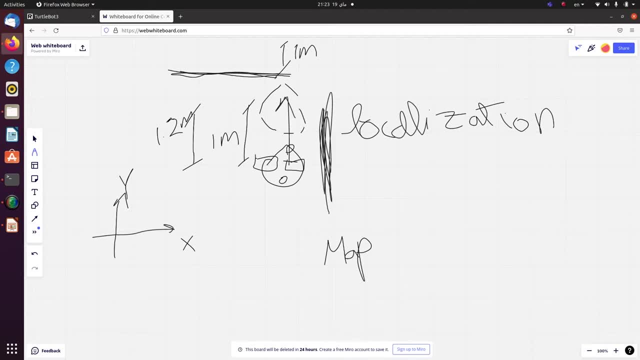 reading of the IMU which says, for example, that he moved 1.2 meters. and we've got the reading. actually, the reading of the lidar itself has some noise embedded into it, but the noise of the lidar is quite small because we call this sensor like an update sensor and update sensors, or update. 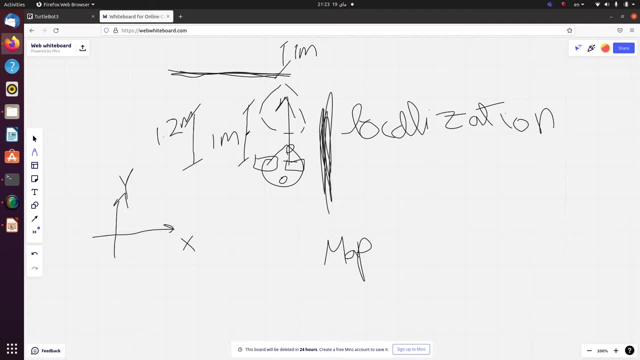 measurements have a high level of accuracy. they have lower frequencies, like I get an update every you know lengthy period of time compared to an IMU. so the IMU gives reading like every, for example, 0.1 second, but the LiDAR would give you, say, an update every one second right. so 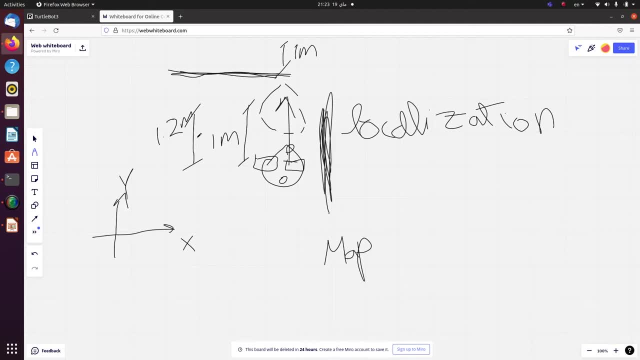 we have a compromise between accuracy and speed or frequency. all right, so it's a compromise of two things. we also have another source of that reckoning, which is the encoders. right, the encoders are sensors that are attached to the wheels and compute how many revolutions did these wheels make? so, by computing the 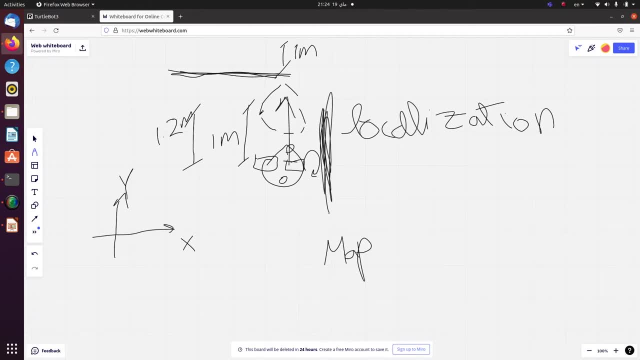 number of revolutions. we can have an estimate of how much we moved, or we can compute the velocity of the or the angular velocity of these wheels, and by integrating the velocity of the wheels, we can compute the velocity of the wheels. we can also have an estimate of how much we moved. using your quarters is better. 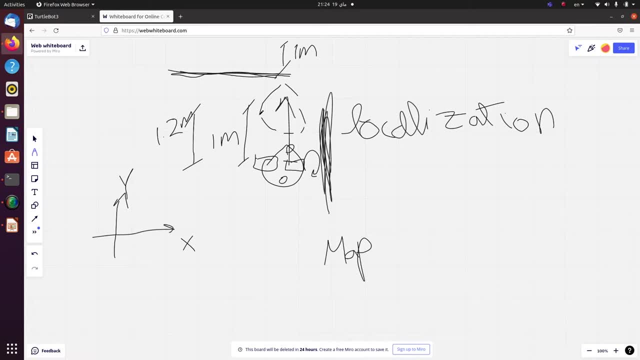 than using the axle at the accelerometer of the IMU, because instead of double integration you only have to do single integration. but still there is some noise embedded into the encoder reading. because the encoder is not a perfect sensor, it will not like compute the number of revolutions very accurately. 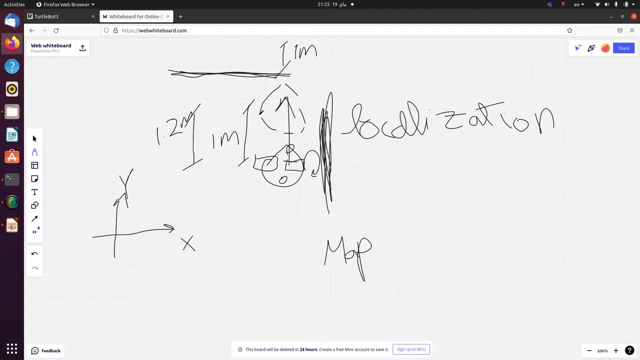 because sometimes the robot is moving too fast and sometimes the sensor like slips some birth counts right. so what we do here, what the localization process includes, is that we compare, for example, the readings from all sets from all sensors against each other and we compare them with the map readings, so we can 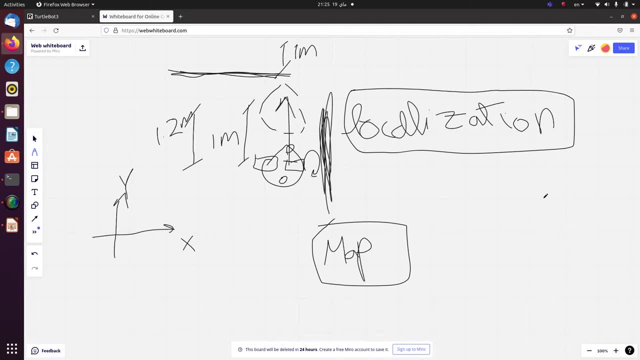 got like the map, which is the source, and sometimes we got something called the prediction. Alright, so what this prediction means is practically any dead reckoning source, and sometimes, when we don't have any prediction sensors, we use the dynamic model of the robot in order to 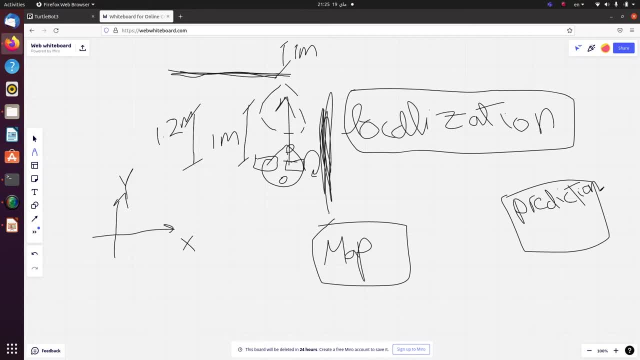 have an idea of where the robot is right now. So by knowing the mass of the robot and by knowing the diameter of the wheels and by knowing the specifications of the DC motors that activate these wheels, I can have an idea of how the robot, or how the dynamic model of the robot works, and then I can have an 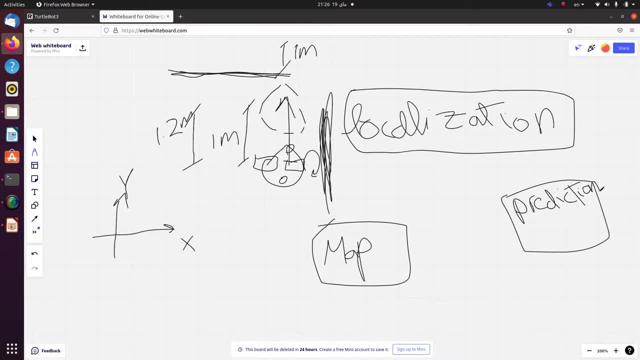 estimation of. for example, if I provided a voltage V for a number or for a, let's say, a specific period of time, t, then I can substitute with these values or I can plug them into the dynamic model and get an estimate of the position of the robot right now. 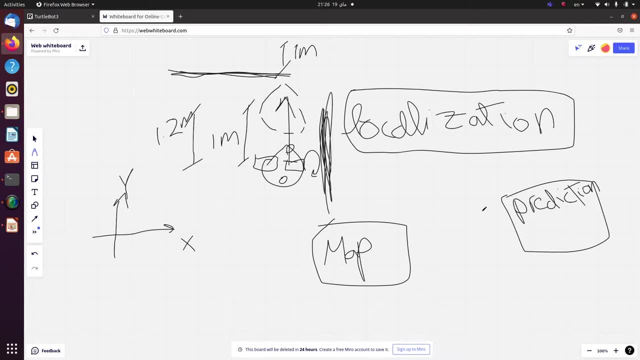 So that's another dead reckoning method. So through information coming from the map and information coming from the prediction, we can have a product which is the location of the robot or the localization of the robot. All right, so localization assumes the presence of a map, so that means that the map is already. 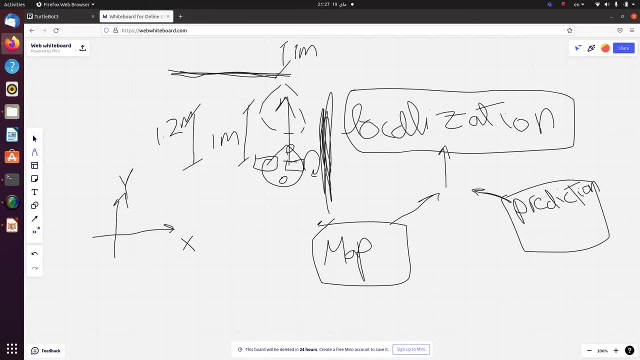 there and the map was drawn in advance. So I'm not like using the lidar in a real-time situation. I've already used the lidar and I've just drawn a map for the entire place or the entire environment, and then I'm using the static map, and by static map I mean a map that was. 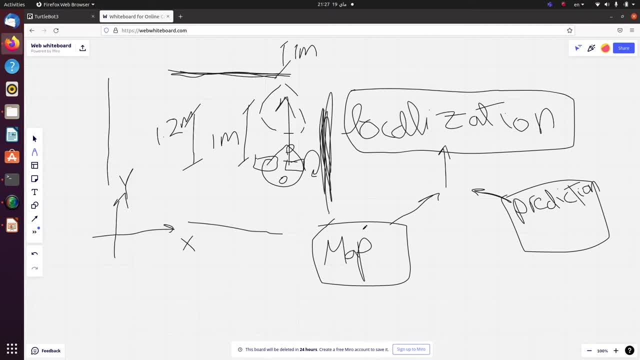 prepared in advance. All right, in order to localize the robot. so by comparing information from the map and information from the prediction right, we can estimate the location of the robot. So this is pure localization And sometimes I might depend only on data coming from the map. say, all right, yeah. 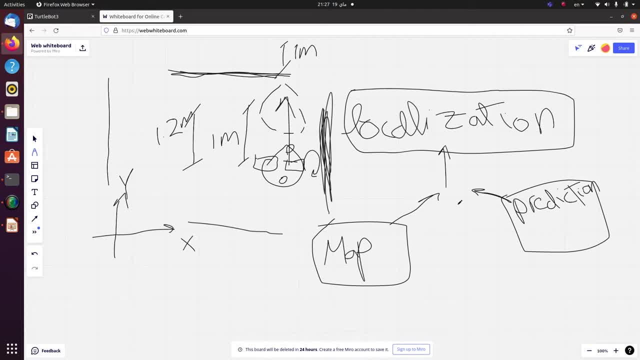 I don't know sometimes. no, it has to be prediction included as well. So by these terms, all right, are used for the localization process or the terms that are involved within the localization process. We have another process called mapping, which is the reverse of what we just said. 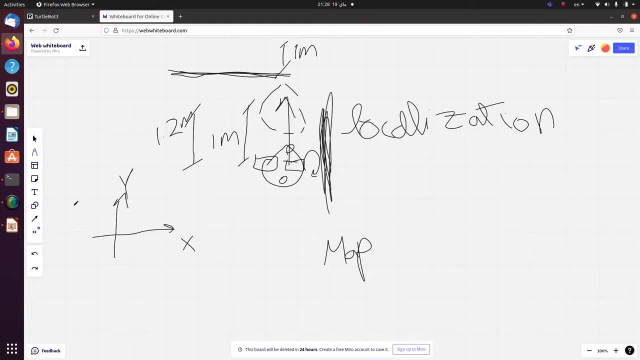 So let's clean up everything Right. Everything assumes that we have the location of the robot in advance, So there's some very accurate sensor that gives us the global location of the robot. All right, Whenever we're moving, we have an accurate estimation of the current location of the. 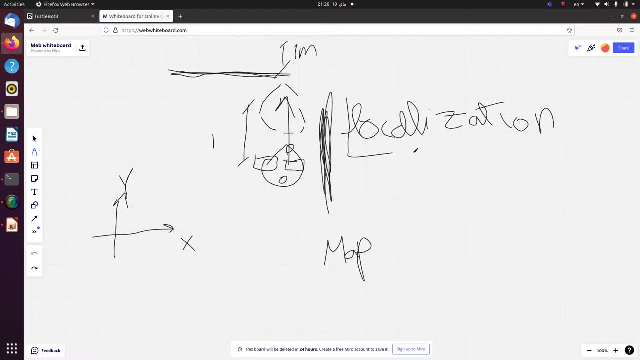 robot. So localization is covered, But actually we don't have a map. All right. So let's just assume we have some sensor like a GPS, And let's assume that this GPS is very accurate. all right. So this GPS gives you an online feedback of your current global pose. all right, without 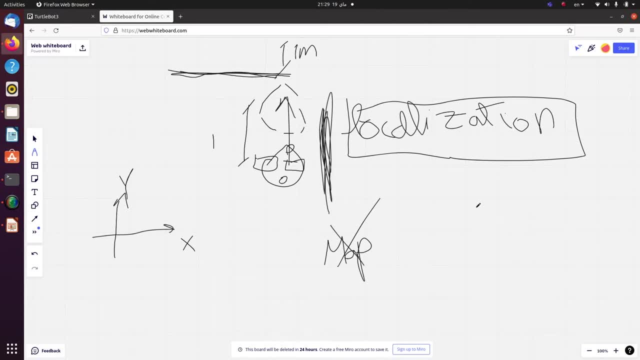 needing a map. So the localization part is covered, But you need to make a map of the environment. You need to map the environment, all right, And this process is called mapping. So we use our LIDAR sensor in order to like have some observations. 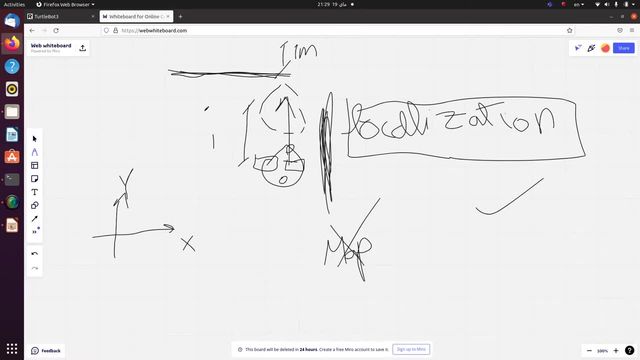 Right. So we're going to like gathering all of these observations during some span of time And we're going to group them together, Right? It's like that shot in the Iron Man movie when Iron Man was showing his design when they were imprisoned in the cave. 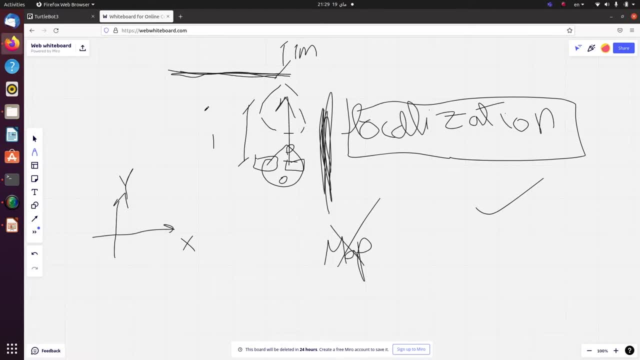 And he was showing his design to the other scientist- I think his name was Jensen, I guess- And what Tony Stark did is that he had multiple drawings or multiple layers of drawings and he had to like overlap them together in order to give the big picture or the entire suit view. all right, 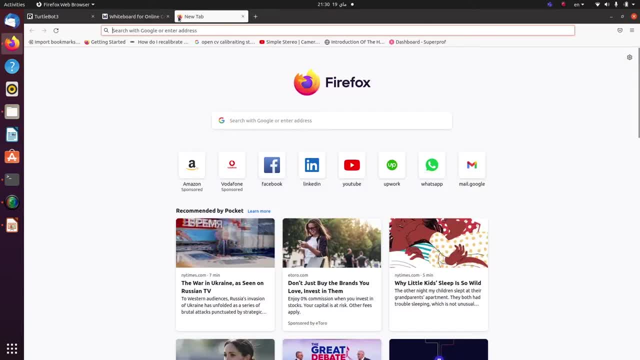 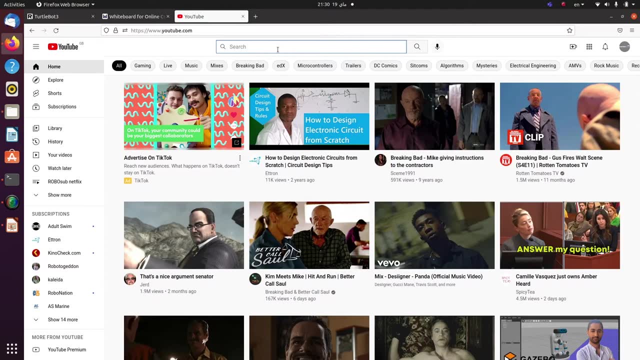 So I don't know if I can get that in YouTube in order to let you have an idea of what I'm trying to say. It's kind of weird, but it will help you understand what I'm trying to say. So let's just say Tony Stark, for example, Mark I. 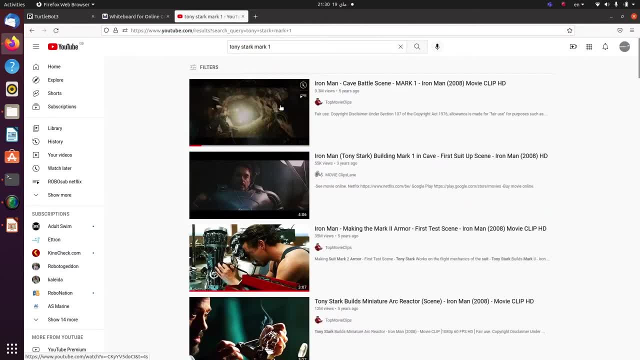 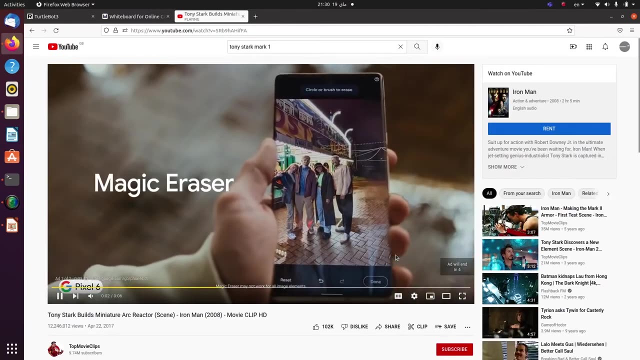 And, yes, I'm a Marvel nerd, right, So I think it was that one. No, not this one. I think it's. yeah, I think it's this one, But of course, ads And other ads. 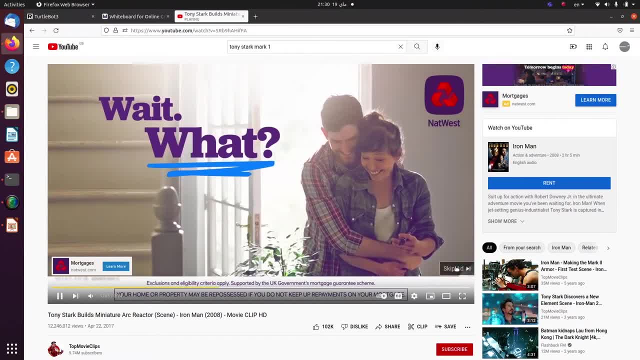 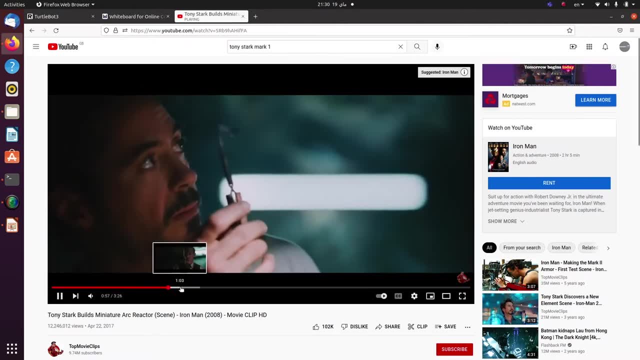 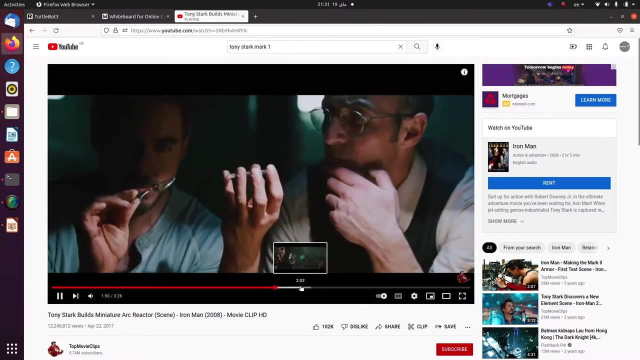 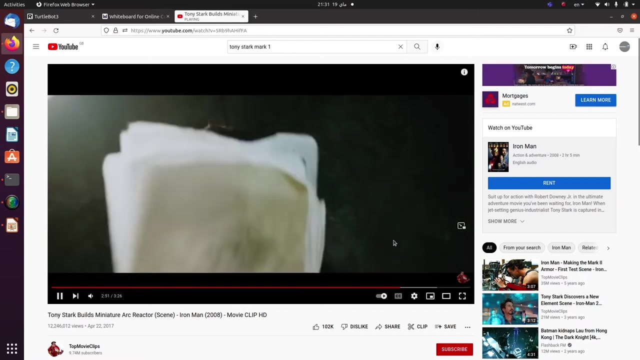 Okay, Cool, Wait what? I hope it's the one, because I don't like ads. All right, so they're working on the arc reactor here and he was trying to power his suit. So yeah, this is where he brings the layouts of his project and he's got like multiple. 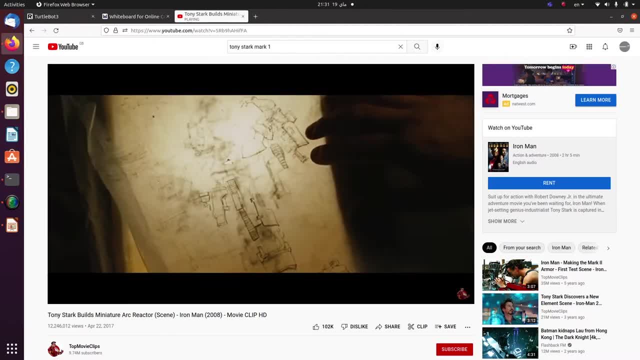 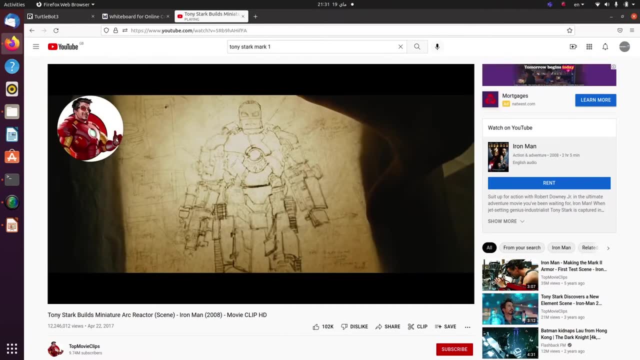 observations, all right, or multiple maps, And he's trying to put them all together, these individual observations at different spans of time, with different robot locations, and he's trying to overlap them together in order to get a full picture. all right. 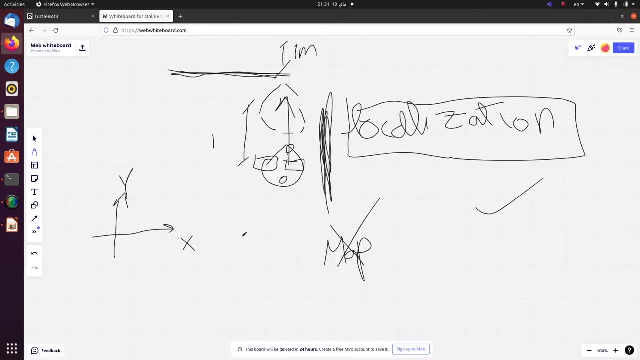 So this scene illustrates what I want to say. So we've got like multiple observations. So let's say that the robot had an observation here. So this observation looks like, for example, if we include it in a separate drawing, then 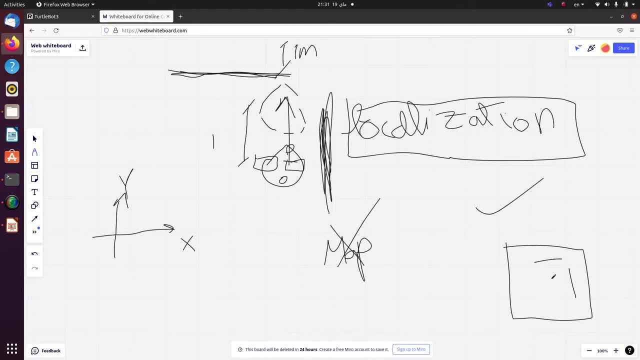 that is the current observation, All right, And the robot location is, for example, you know, here, for example, here. So let's just say that the robot moved here with its face having an angle theta like that, so its face is like this. 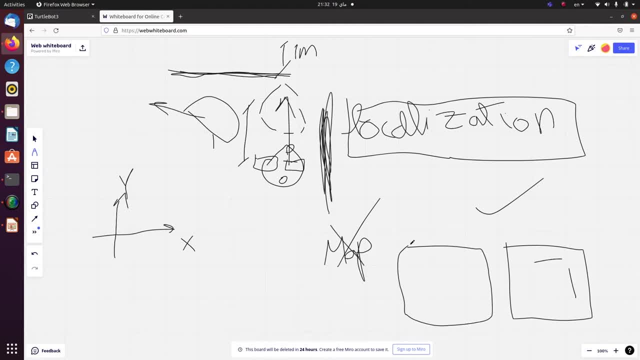 So we will have another observation And since this robot now represents the center of my individual observation, so I'll get like an observation which looks like that, Like, for example, something like Okay, Something like this And something at my back. 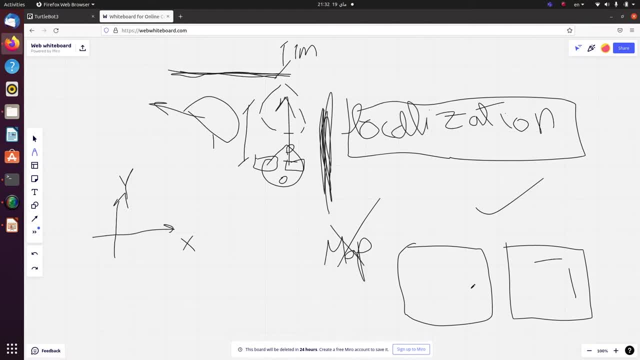 Maybe it will look a little bit like if I'm facing the robot like this, so we'll have something like this maybe. Yeah, it will be something like this. all right, And I move forward again and I move like here: 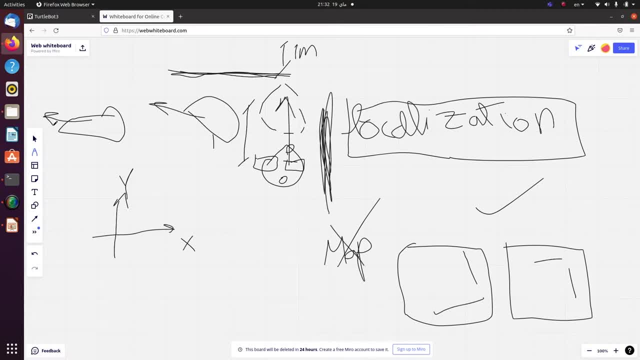 Sorry. So the face of the robot is here and I get a third observation, all right, where the robot is basically like having an observation which looks like this right. So for each one of these observations I got a record of the robot location. 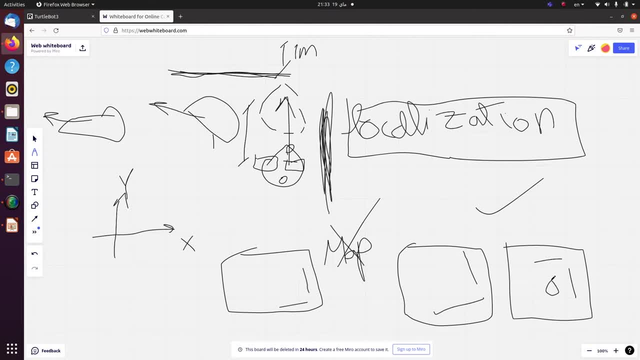 So I know that the robot here was like looking that way, and I know that here the robot was looking somewhere like this, Okay, A little bit rotated, and here the robot was looking here, for example, right, So by, like, by overlapping the robot locations in each of these observations, so I get all 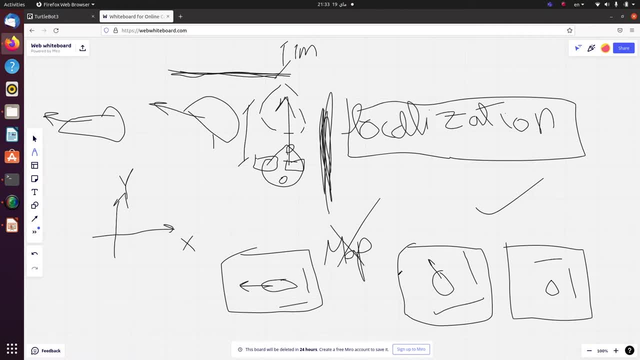 of these images, or all of these individual local maps, and I overlap them together in order to get a very strong map where, for example, this is the The robot pose after overlapping. so I got all the robot poses to overlap together into 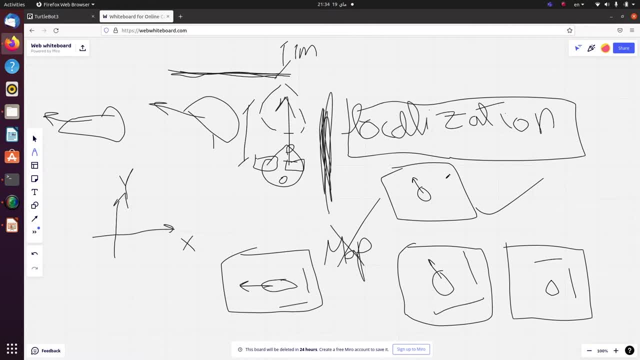 you know a single entity here, and then I get a very strong right. I get a very strong like drawing, or a very strong belief in the location, or the location of the obstacles. So too many obstacles are overlapped together. and then I know for sure that the global map. 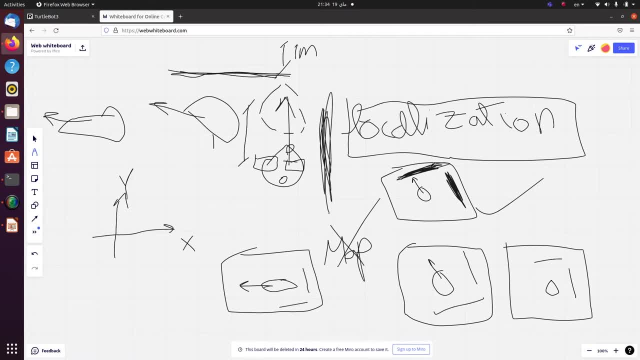 has the obstacles, for example, here. all right. So this is what mapping is all about, and it assumes that localization is covered. So you either have localization covered and mapping missing, or mapping is missing and you need to have localization active or have a localization module. 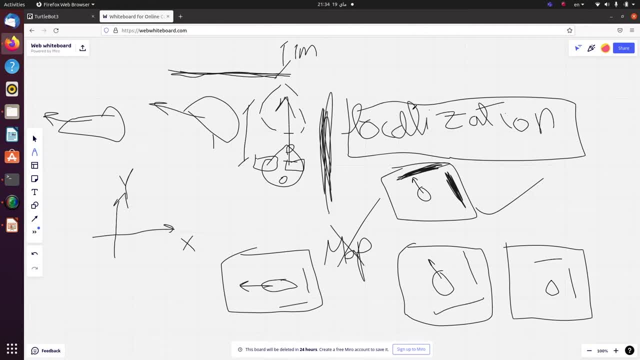 So what if I'm navigating through an environment that I know nothing about and, at the same time, I don't know where my robot is? I had an idea where I placed him, where I placed it initially, but I don't know where. 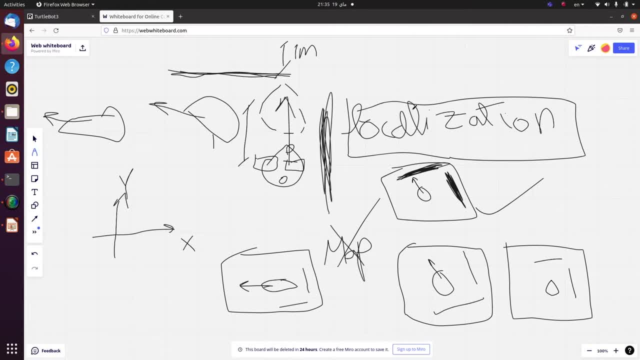 the robot is heading right now. So this is called a problem of SLAM, which is short for simultaneous localization and mapping. So let me just paste some stuff. And the problem of SLAM is a complex problem Because you're trying to, you know, get localization from mapping which does not exist, and 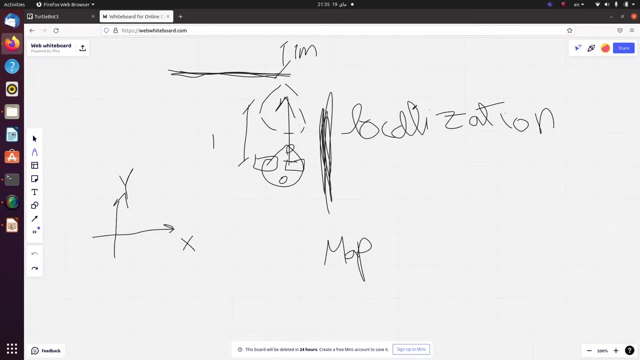 get mapping from localization, which also does not exist. So this is crazy And it's a complex subject that would require, you know, a separate lecture on its own. But let's just say that by fusing the data coming from different sensors, we could obtain: 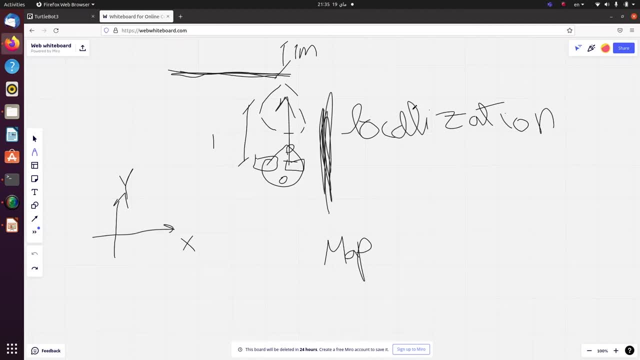 what you can say is: you know, a sensor fusion, Right, And we can say that it's possible. right, It's possible. let's say that, you know, if you're trying to do a map, you can see the map, right. 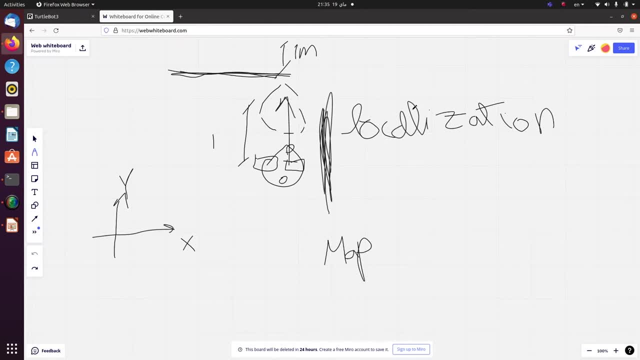 Let's say you're trying to do a map and you can see the map as a paradigm and you can determine the pose of the robot right, Maybe not accurate at first, because you're trying to construct the map and your localization belief at the same time. 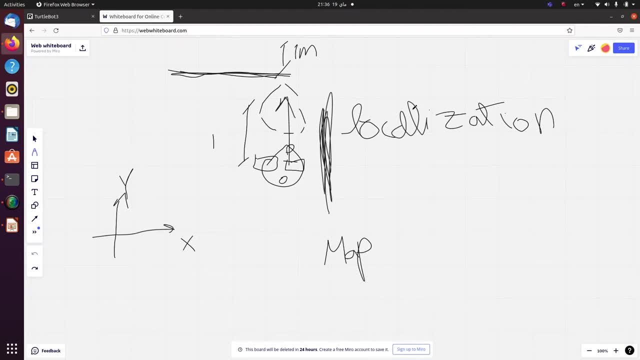 So they're both going to depend on each other or rely on each other And they're both like quite vague at the beginning. So you'll start with a pretty low accuracy. then you will converge eventually to a strong belief, unlike the other paradigms: localization or individual localization, individual mapping. 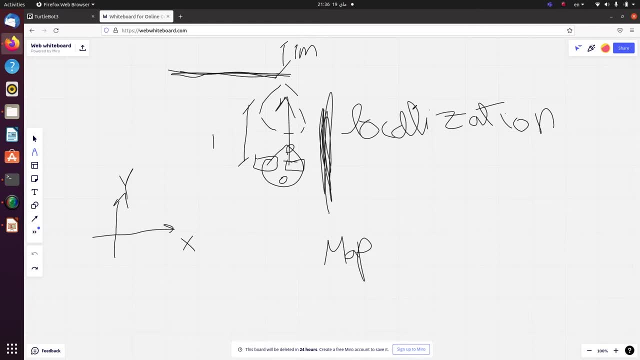 you start from nothing and you try to build both beliefs- which is the pose belief or the localization belief and the mapping belief- at the same time. so it's going to be quite poor in the beginning, and then you try to improve the localization accuracy and the mapping accuracy. 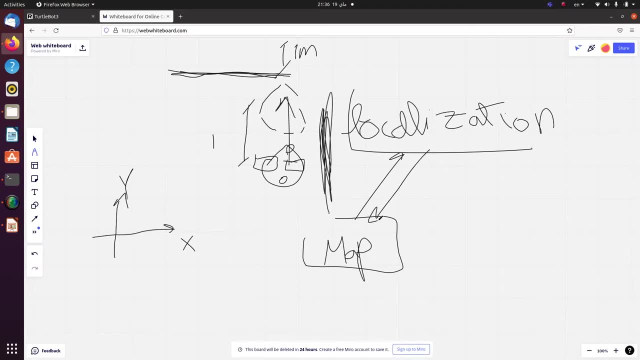 by making them rely on each other, so they both support each other. once you have a new information, that could, you know, improve the map. that will simultaneously improve the localization. so let's have an example where the robot is navigating and we've got our set of sensors. 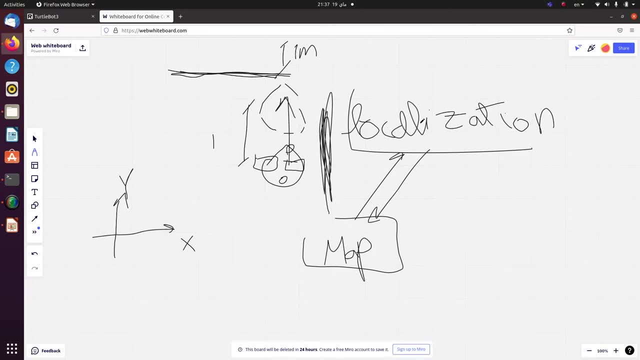 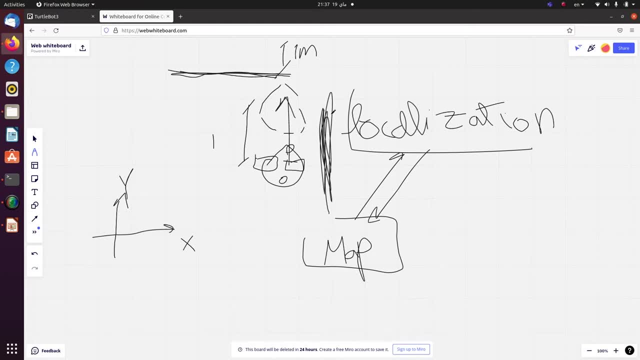 you take a shot and or a lidar shot so you get like a local map right that's attached to the current location. all right, the current location is unknown. so i just say that the current location, which was unknown, had a local map, for example with this: um lidar shot, all right, so later you will. 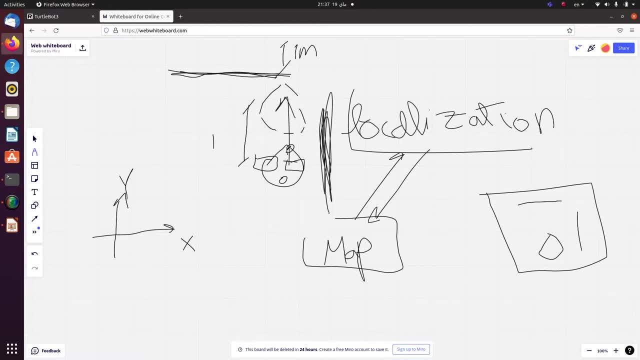 all right, you will have some prediction of where you're are now. so you'll say that, according to my dead reckoning sensors, i moved like one meter, all right, and this one meter is quite noisy, all right, but it's the best estimate i have so far. 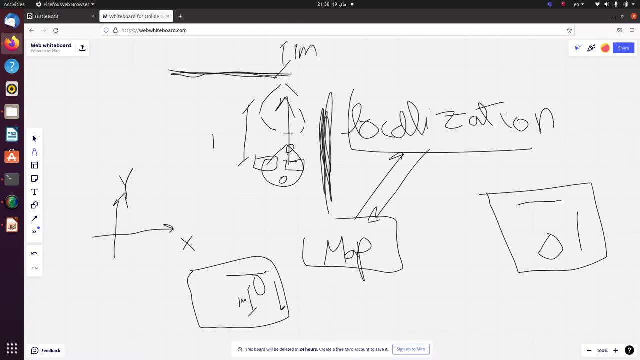 and then i had another shot here which indicates that this uh wall is now at a distance of like 0.9 meters, which means that i most likely moved a distance which is which lies between 0.9 and 0.9 and 1 right. so through some sensor fusion paradigm, i can now say that the robot moved. 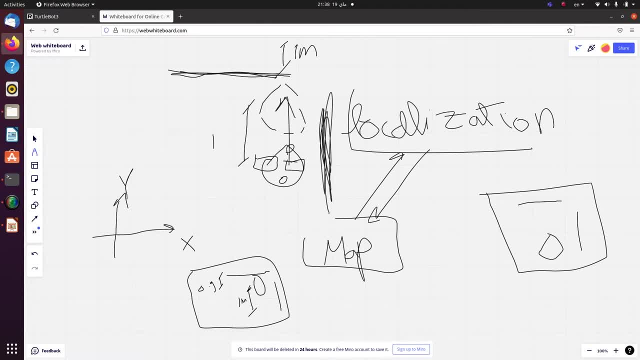 a distance, all right, which with an estimate that is better than both the individual reading of the lidar and the individual reading of the uh dead reckoning sensors. so i'd say that i moved like 0.95 meters, for example, relative to my first location, right, so i begin to denote my first. 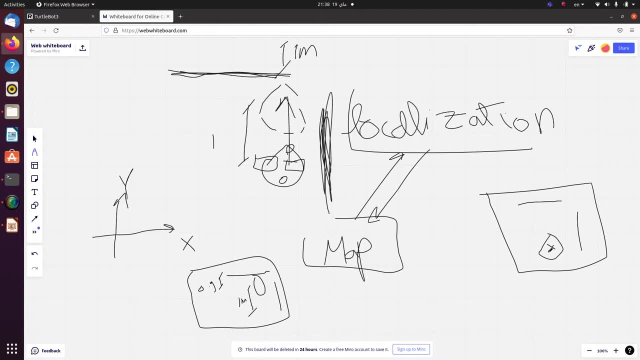 location, as you know, um the center of the global map. i'm trying to uh develop and i'd say that i moved one meter or 0.95 meters from that particular location, all right. and since i moved 0.95 meters from that particular location, all right, so i got a new location. so the mapping process kind of intervened. 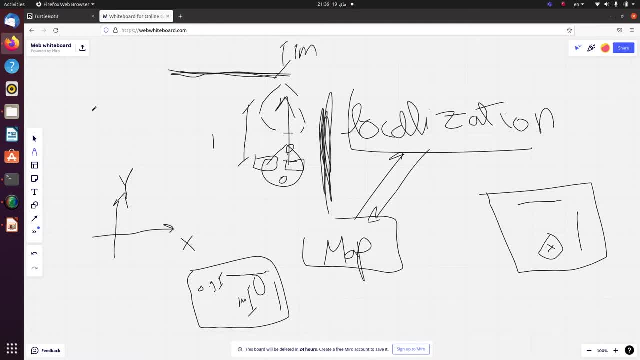 with the localization problem, but i still don't have quite a global map. i just constructed a part of the environment according to my current observations. so let's just say that my entire map was something like that and i just, you know, mapped a small part of the environment, the 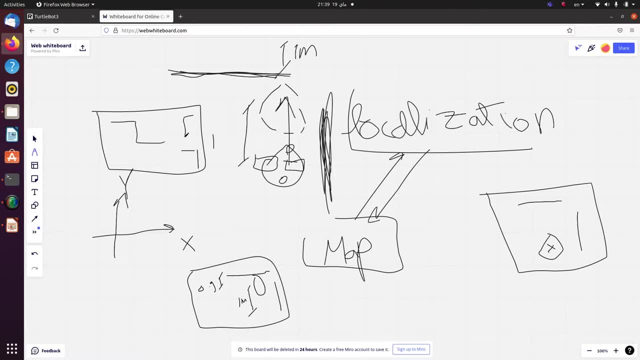 environment would actually look like something like this, for example: right, but i just mapped that part for now, so this is like a partial map. so whenever i keep going, all right, my localization sensors could help me, like, determine where the new uh obstacles are. so if i know that, for example, i moved right here, so my new local map says that i moved, like, 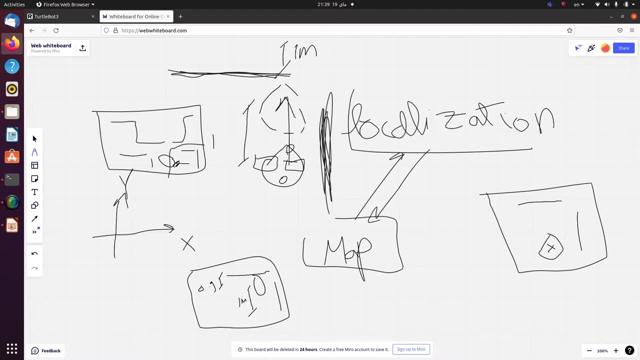 for example, a distance of 0.5 meters to the left, and i rotate it with a theta that is equal to, for example, that makes like 120 degrees, for example. right, then i got a new shot, and this new shot looks like something like that, for example: 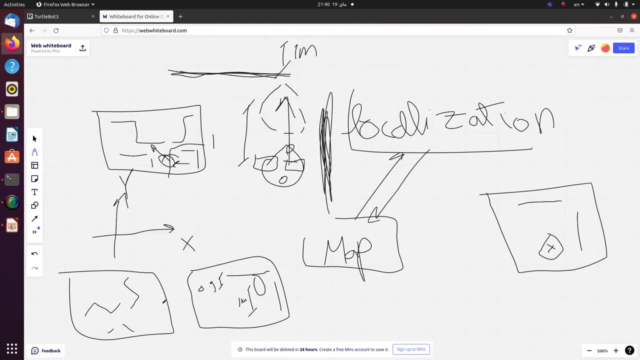 right and i know that, um, my old observation was this shot, for example. so my localization module, or the localization part of my algorithm, now said that i moved, like uh, 0.5 meters to the left and rotate it with, for example, 120 degrees. so based on this localization data, i can like reorient. 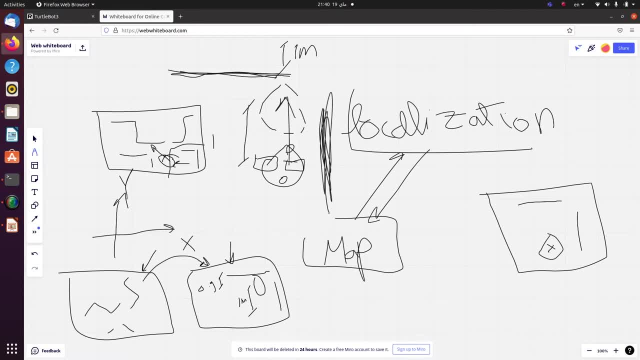 the new observation to you know, map it to my global map, all right. so i've got a local map, which is the local observation. i got some global map that i keep building through individual observations. so in the global map the first observation was recorded right here and according to this new 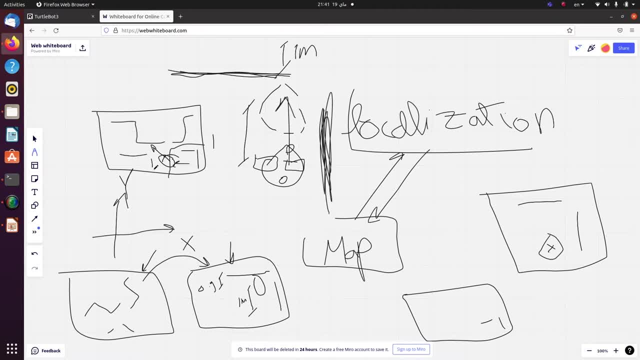 observation and according to the localization data i got so far, then i can deduce that indeed, this observation can be mapped to the global map to be somewhere here which kind of matches what the actual physical map looks like. all right, so i'll continue building this map and localizing myself, and the more i localize myself, 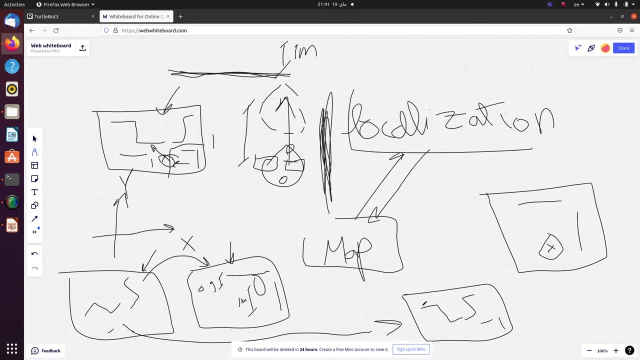 and the more i map the environment, then my belief in both localization and mapping will grow stronger. all right, and this is a pretty, you know, intuitive understanding of what's going on, because actually this is a pretty complex algorithm that is on probability distributions and you know something called particle filter. 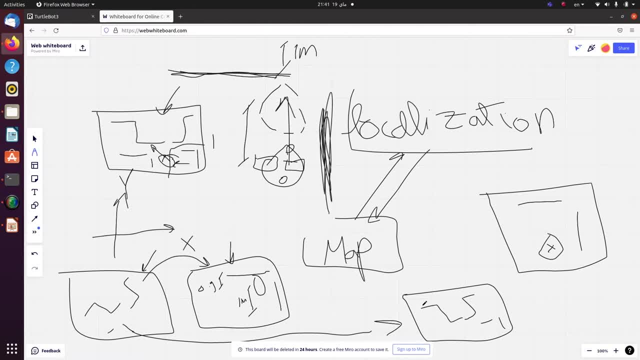 and we'll go through that. right. but right now we'll just do with what we have so far and we'll try to implement those algorithms in gazebo simulations. in fact, we're not going to write the algorithm ourself. it was already written by some Ross developer who was working in some R&D department. right, what we're? 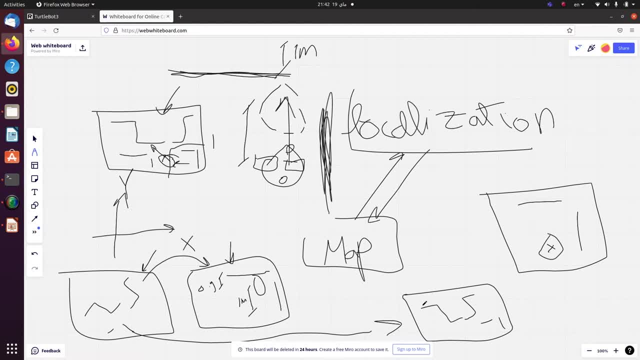 going to do as engineers now. we're going to like implement that without having to know what the black box includes. we can have a simple idea of what was going on, but the details of what's going on and the entire mathematics behind the stuff can be explained in another course. 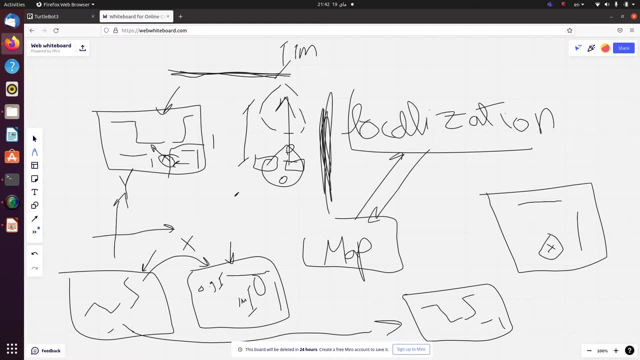 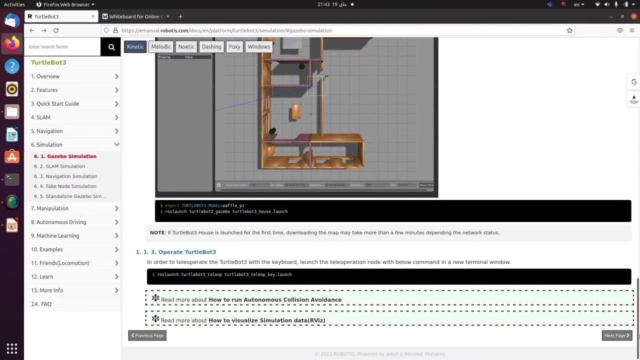 right, so that's the end of that part, and we're going to explain more as we're progressing through the simulation itself. so I got back here to my e-manual. this is the page that we finished and we're going to head to the next page. 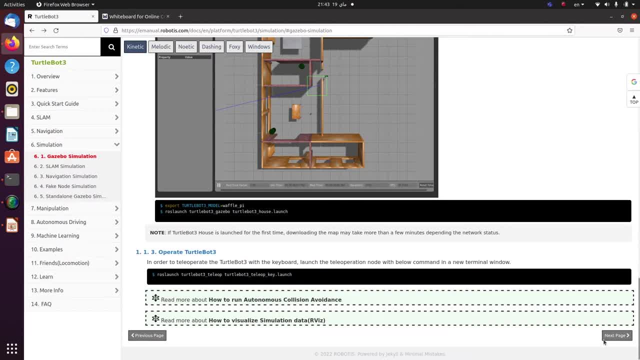 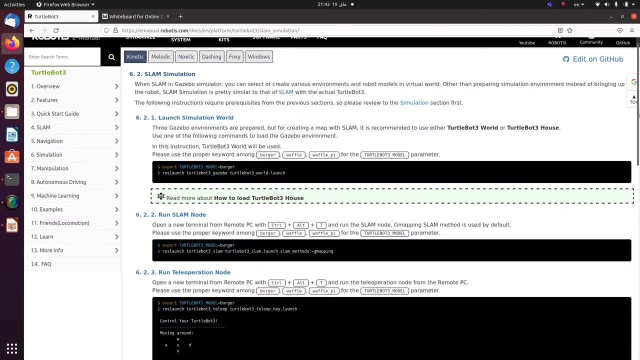 which includes the SLAM simulation. alright, so here we're on the SLAM simulation page. so the SLAM, as we said, is the Simultaneous localization and mapping feature. all right, and there are multiple algorithms that you know Do slam, right. so slam is not like one algorithm, It's a family of algorithms that. 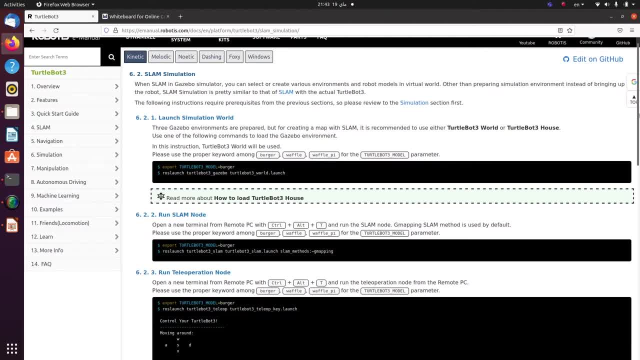 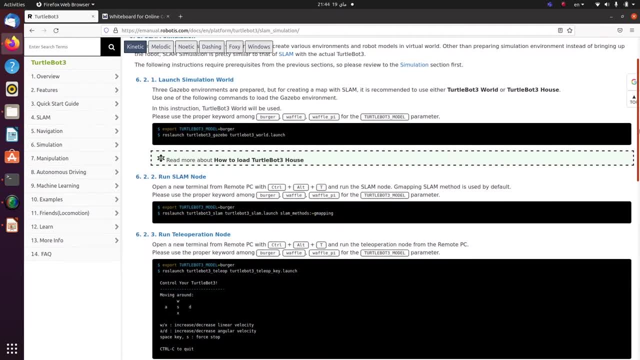 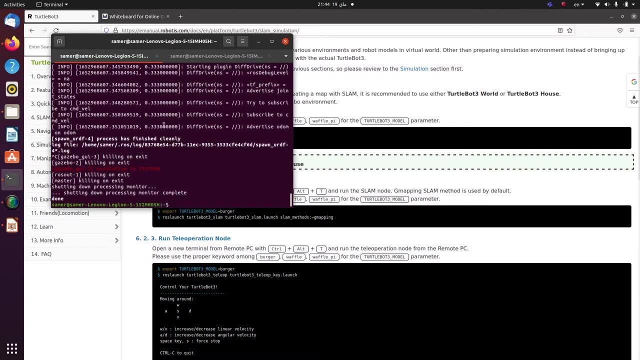 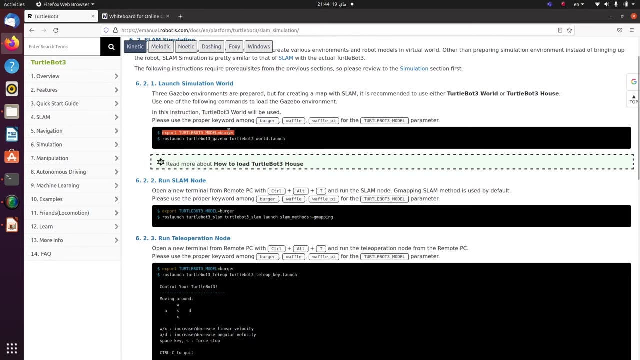 Do or does simultaneous localization and mapping right. So, first of all, I'm going to launch my or spawn my turtle burger Into a turtle bar three world. so I'm going to open up my terminal here and I'm going to export the model, which is burger for now. so I'm going to copy that. 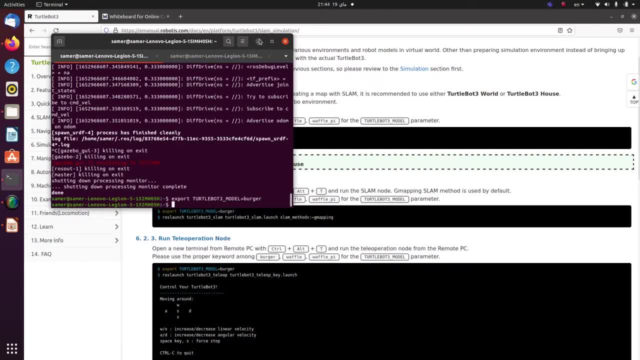 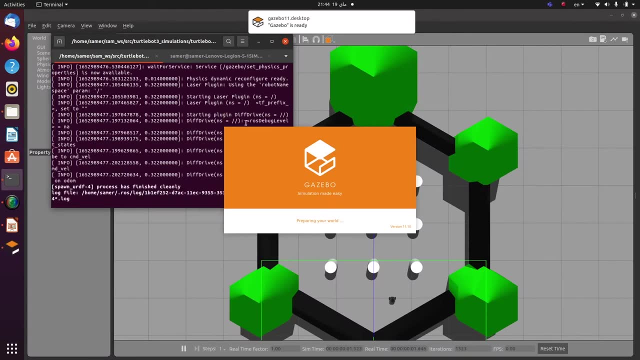 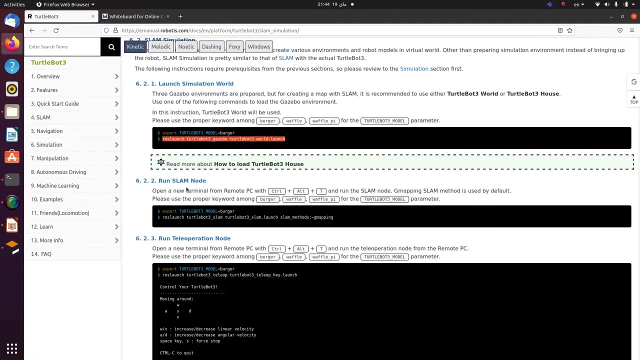 I'm going to paste here. Then I'm going to launch my turtle bar three world. I'm going to paste that here and Again. if you're running this for the first time, it's going to take a little longer than it did here. All right, so this is my environment. what we need to do now is to run the slam note. 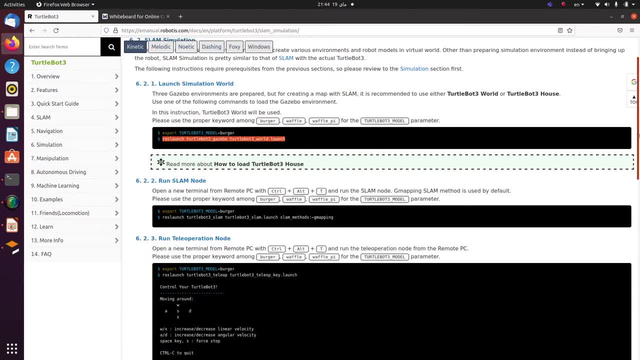 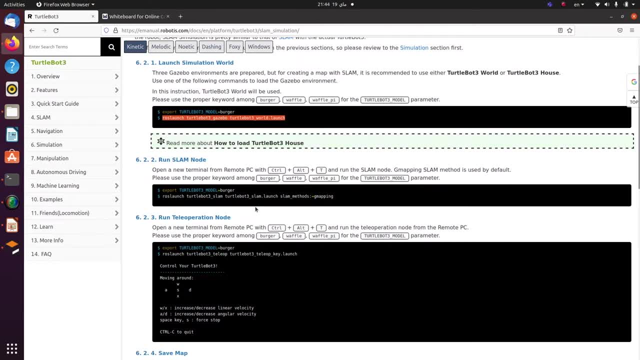 All right. so in order to run the slam node, We need to open up a new tab in our terminal and We also need to redefine our total bar three model, because that variable is like tab specific. so whenever you open up a new tab, you have to redefine it, and 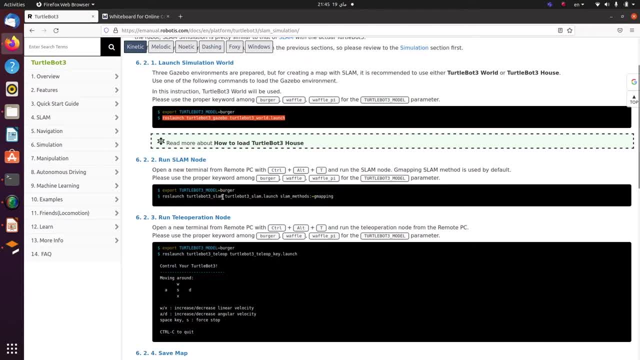 You will launch the total bar three slam package and you're going to launch a story. You're going to, you know, run a certain file called to the bar three a, slam The launch and you're going to determine your slam method to be g mapping method. there are other methods. 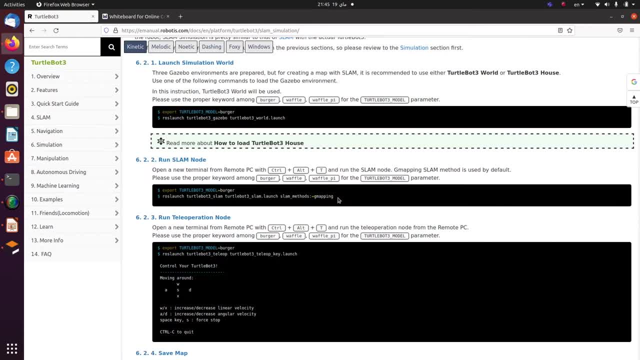 But the g mapping method is one of the most famous methods and one of the most widely used methods, So it's like the standard method for most Ross developers, So we're going to go with that, Alright. so, first of all, as we are, we are navigating through this. 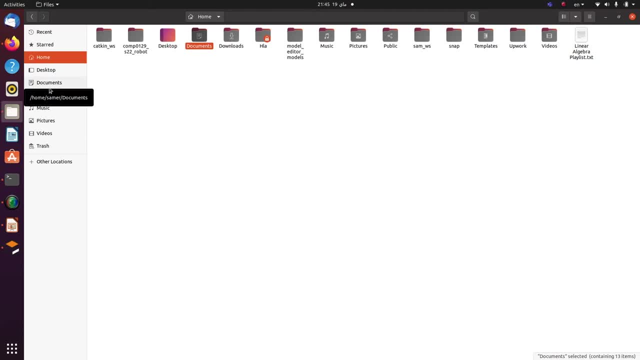 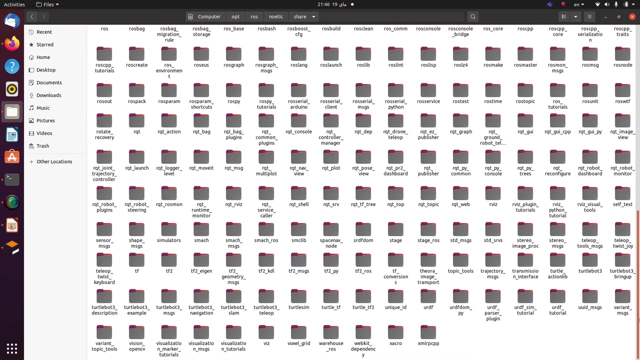 Package? all right, we need to, you know, look through its details. so I'm going to head to the other locations- computer, opt, Ross, Yannick and the share file which includes all the packages, and then I'm going to look for that turtle, sim slam or 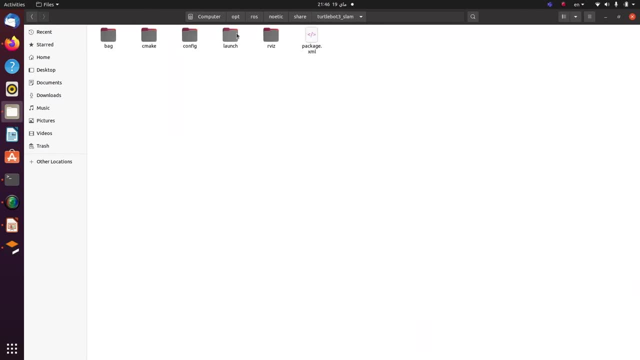 or total bar three slam, sorry. So we've got a number of files. We got a launch file here, Right, and you can find here that there are multiple slam methods. So we've got the Hector method, for example. you've got the card which is, which I think is short for cartographer. 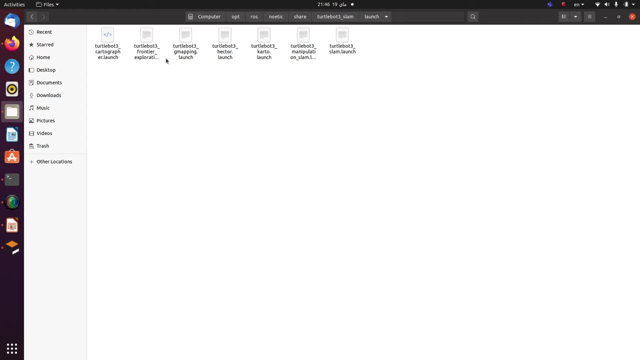 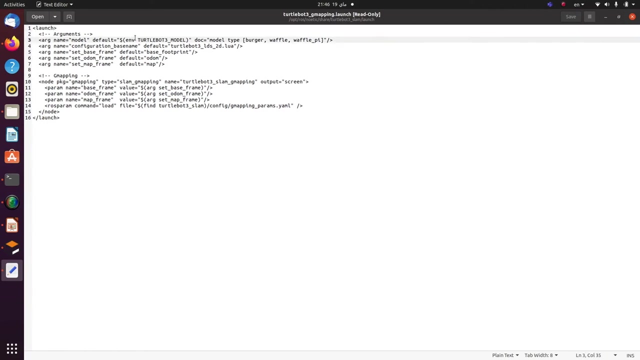 Right, and you've got frontier exploration here. Yeah, here's cartographer, cartographer, alright, so So we're going to go with the gmapping package or the gmapping launch file, So you've got to have a parameter. This is why we need to determine the TurtlePath3 model here. 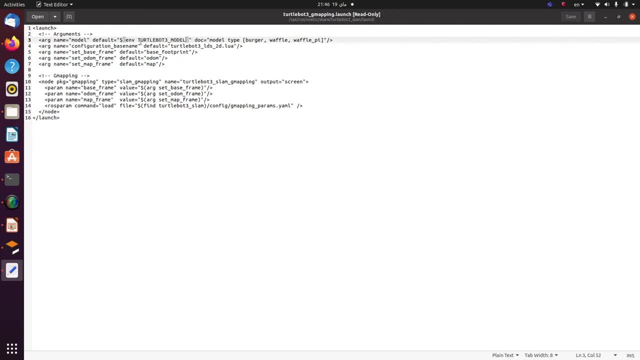 because it's a variable here, So that variable has to be defined in our terminal before we launch this file. And someone might ask: why am I launching this or why am I choosing my robot model? What does this have to do with the SLAM problem? 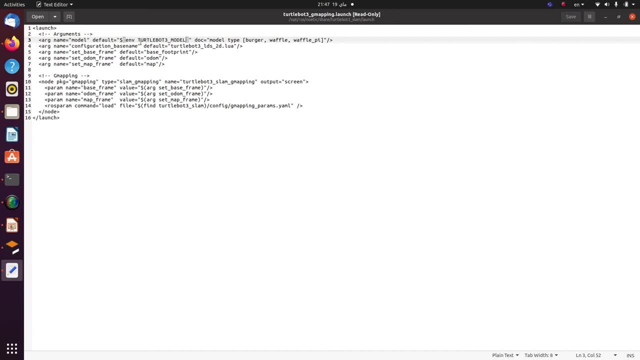 So a short answer to this is that you have a LIDAR and the LIDAR can be attached to several locations or one of different locations on the chassis or the body of the robot. So that differs according to the mechanical design of the robot. 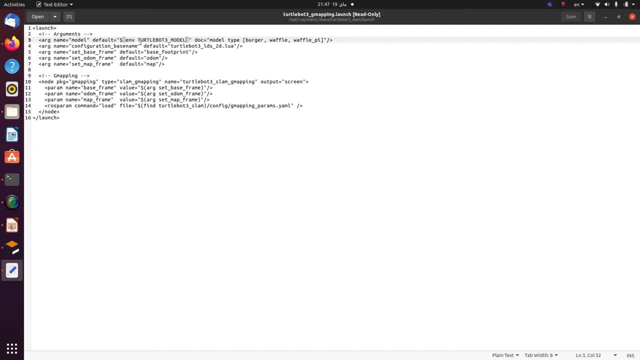 So the location of the LIDAR and its distance from the robot origin is different for each robot, So you've got geometrical differences. So you need to determine your model in order to have the proper transform that's going to be used in your model. 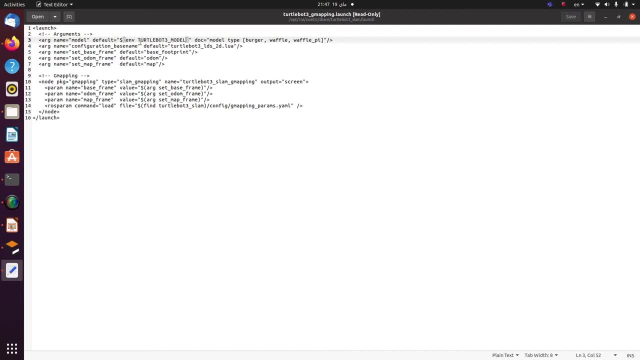 It's going to transform the LIDAR readings, which are a reference to the origin of the LIDAR itself, or the frame of the LIDAR itself, to the frame of the robot. So the LIDAR frame does not have to be coincident with the robot frame. 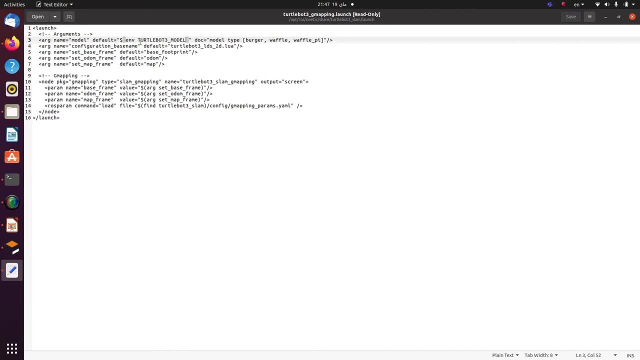 And this is one of the differences that you have to bear in mind- And you're going to set something called the base frame, and the base frame is basically, you know, it's like the origin, It's like the origin of your robot. 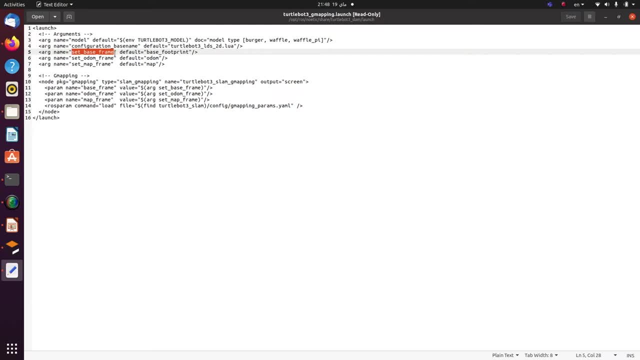 Your robot has some local frame or some body frame, as we said before, And this local frame is attached to some origin located you know somewhere in the body. All right, So this has to be determined And you've got the odometry frame and the map frame. 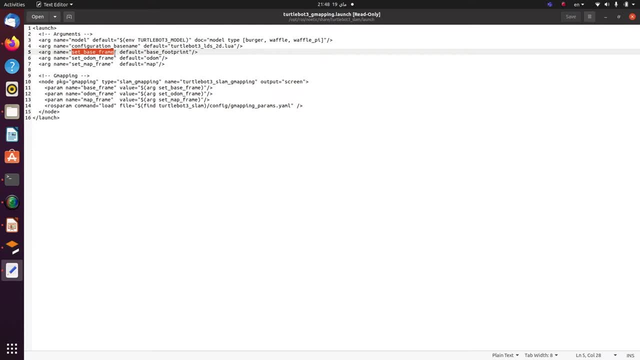 So the map frame is like the global map frame, All right, And the odometry frame is well where your odometry sensors are. So basically, for example, if you have like an encoder, and this encoder is producing, like you know, some readings, 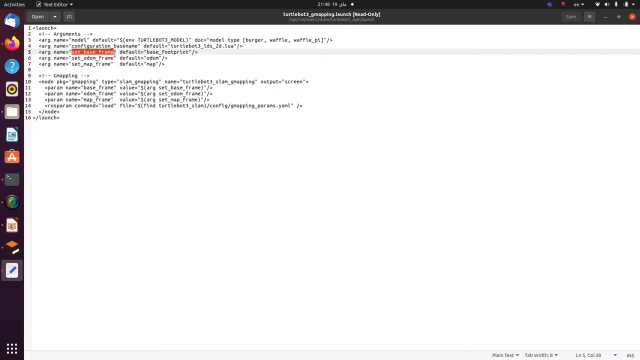 and you're converting these readings. all right, you know reference to some frame. you have to determine the exact transform between the odometry frame and the base frame, All right, So you have to define the frame of each sensor, all right. 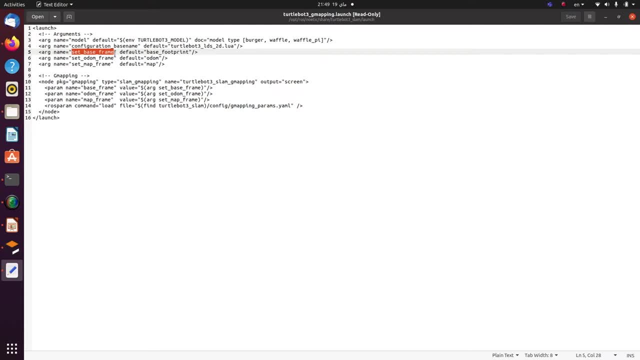 And you've got to relate them to the base frame, because eventually you need to reference everything to the base frame of the robot, not the individual sensors but the base frame itself, so that we can have all the readings consistent and reference to the same local frame. 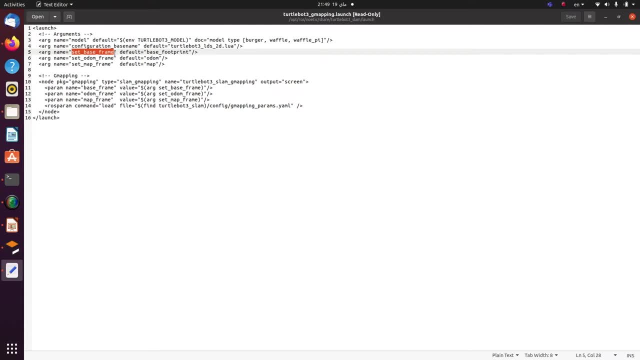 All right, And then we're going to compare this local frame again with the global map frame. So there are a lot of frames and we need to define the relationships between all of them. All right, So this is basically the same thing. 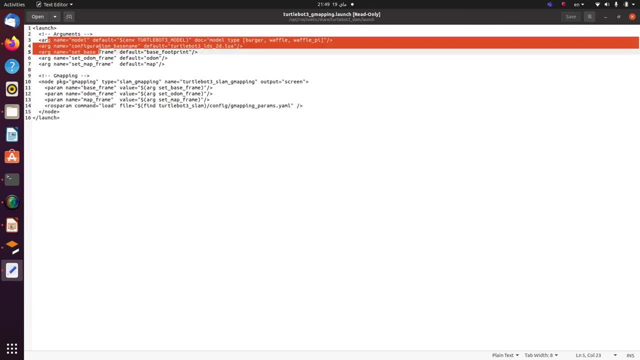 We're just launching the node, All right. So this is basically the same thing: We're just launching the node And, if you want to see what's going on here, we're just determining the values. Here, the values are provided, all right. 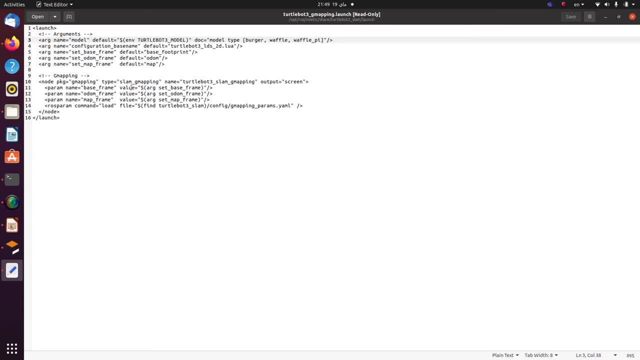 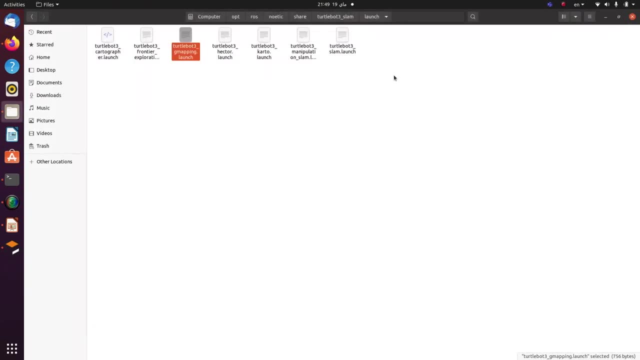 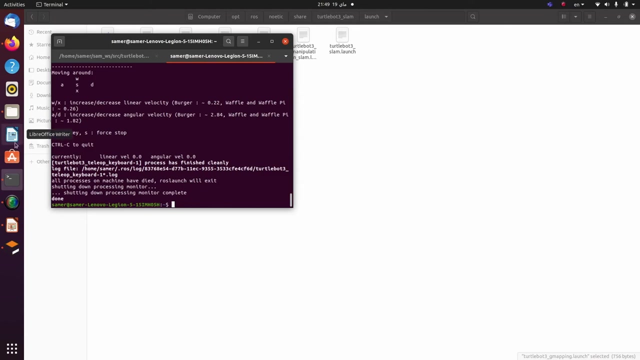 Whether from the terminal or here in the launch file itself, then we're using these arguments or these parameters and feeding them to the algorithm itself before launching it. So that's pretty cool so far. So let's launch it now. So we need to, as I said before, we need to open up, yeah, run the slam nodes. 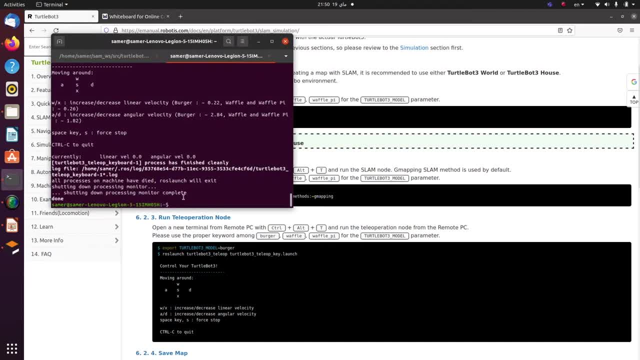 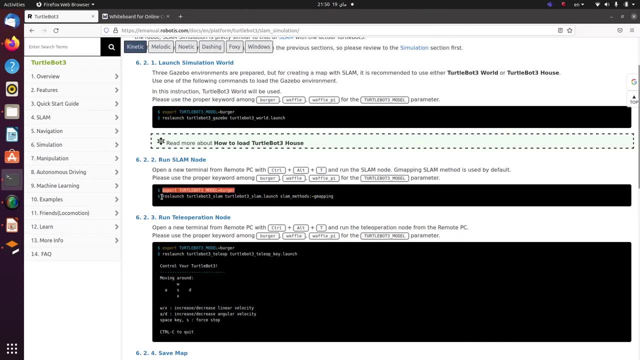 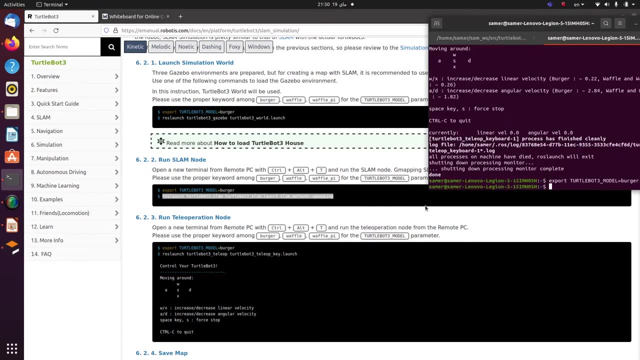 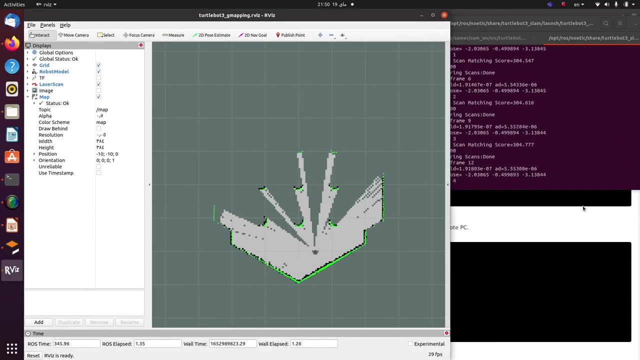 We need to copy that first, And then we're going to run the slam node here, And, as I said before, the slam node means that you're localizing yourself, at the same time constructing a map. All right, now we got something called Arviz that popped up. 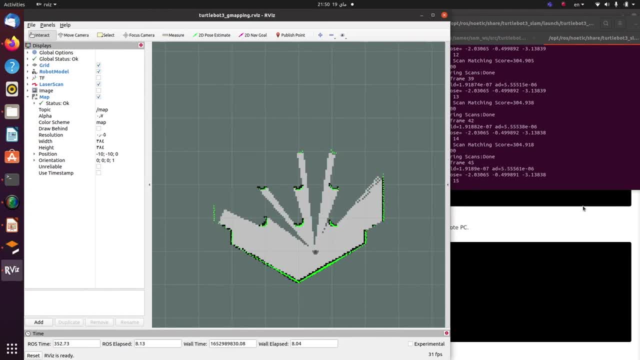 So what is Arviz? Arviz is like a visualization tool That, apart from the Gazebo simulation itself, shows some particular aspects like the readings of your sensors. So I got readings here. these green readings here, I guess, represent the readings, or the current readings, of my LiDAR. 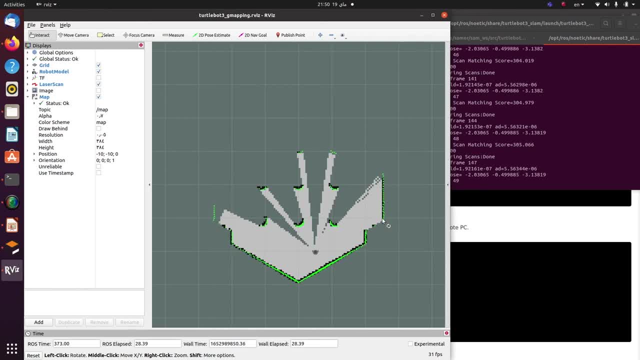 So these are like the ends or the tip of the beam, right. So we've got some displays here that represent, for example, the laser scans. So if I uncheck that so you find that the laser scans, you can see that the laser beams disappeared. 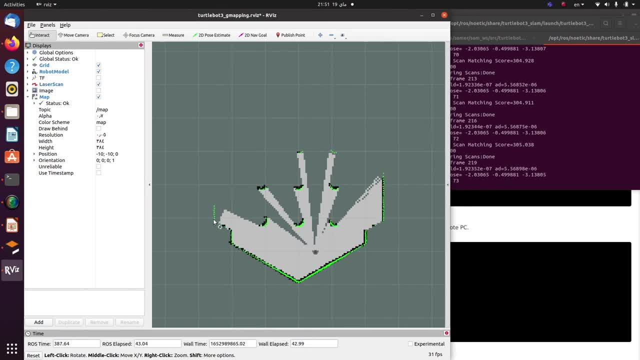 So, by rechecking that, we can find the laser beams that are currently, you know, bursting out of the robot And we can find the global map. So the global map, or the current global map, because this is a global map that is, you know, drawn by the robot itself- 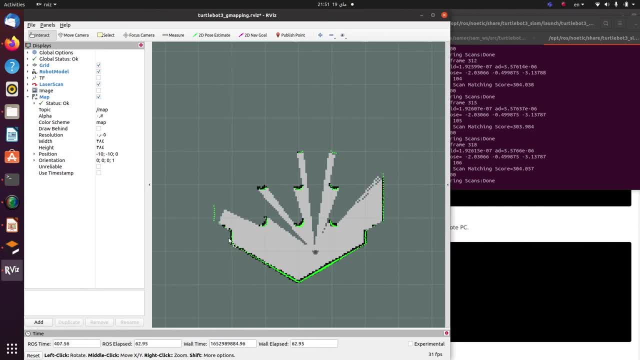 It's not the actual physical map, because the actual physical map would include everything in my environment. So this is the global map that is, you know, currently constructed by the robot, so far. So once the robot starts to move and it, you know, gathers some more information or some more observations. 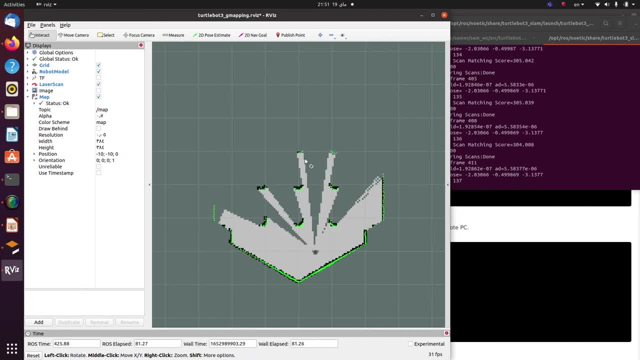 this global map is going to evolve and it's going to include more details, But since the robot is static here, we only get to draw some part of the map, which is the part that is, you know, included in our current observation. 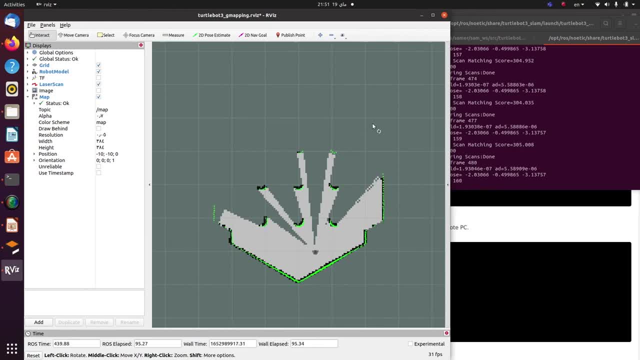 Our LiDAR has a limit, so we can't like map the entire environment using LiDAR uh beams while we're static or sitting at some position without moving. We need to navigate through this environment in order to get more observations and 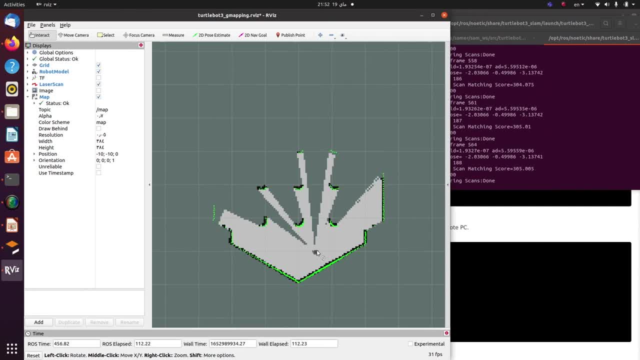 you know, help construct the map or the global map of the robot. All right, So this is basically our vis, and it's a pretty good visualization tool. It lets you, like, have an idea about what's going on. Um, maybe better than Gazebo itself, because Gazebo does not show. 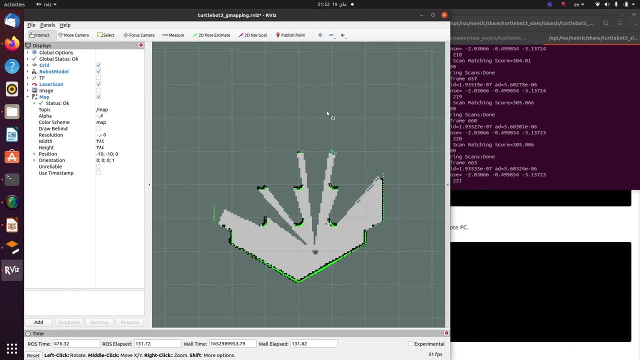 you know, sensor readings, For example, it just shows like a camera view of your environment. So you get to see what's happening, what would happen in the real world when you run this package right. But you know, our vis is more of a troubleshooting tool. 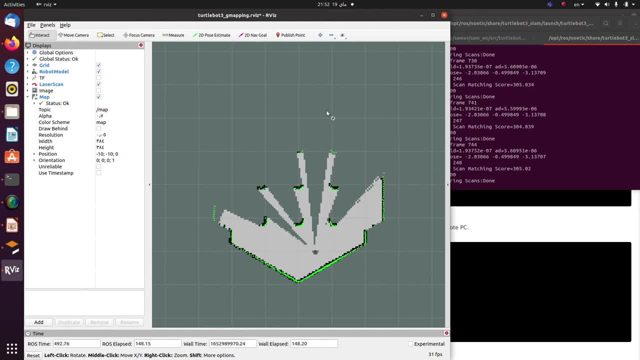 It lets you see the underlying layers, the sensor readings and the current global map that is currently being drawn into the algorithm. So, when it comes to the algorithm itself, you'll find that this global map is actually some sort of a matrix, And when you look at the matrix, 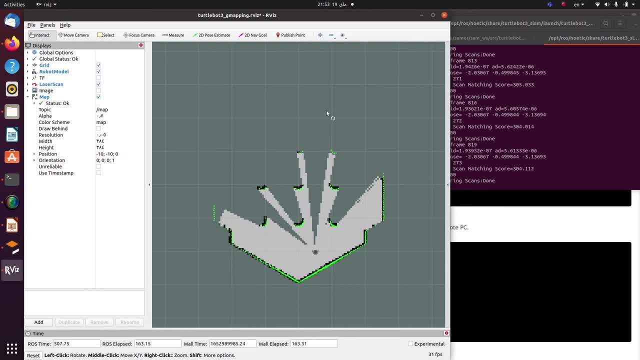 it's. you know you can type it on the terminal, but again it would look like you're the matrix operator that is just there and reading some green symbols and it's pretty hard to interpret these symbols. So our vis is quite useful when it comes to visualizing this global map. 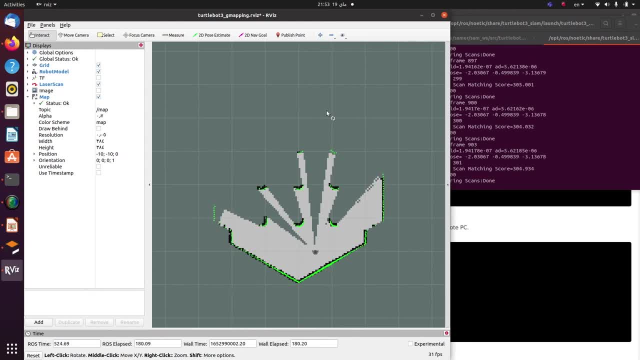 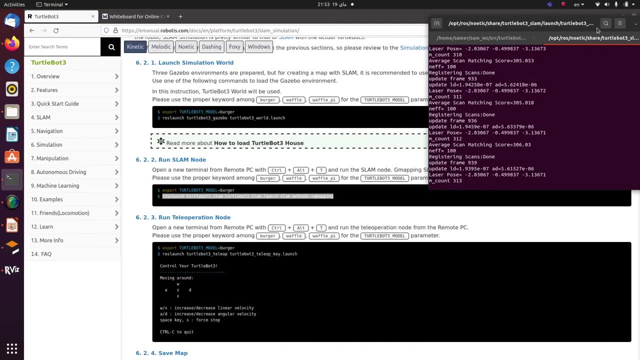 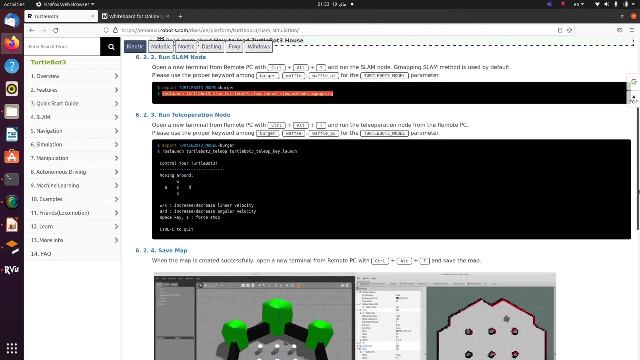 for example, and it lets your task become much easier. You can troubleshoot something that you can actually see and interpret with your own eyes. All right, So let's move on now. We ran the SLAM node, So right now, as I said, 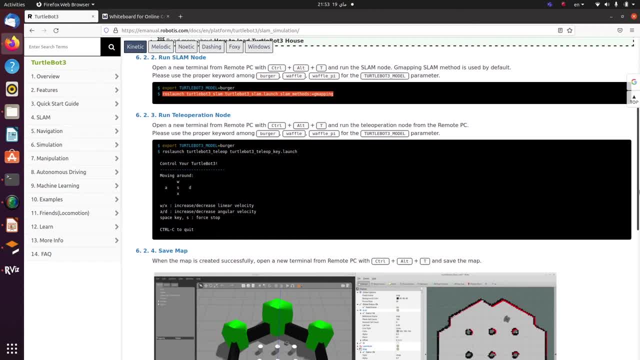 we need to navigate through the environment in order to make use of the G mapping algorithm and start to have newer observations and begin to overlap these observations with the already existing observation and begin to, like, build the global map bit by bit. All right, So I'm going to open up a new tab. 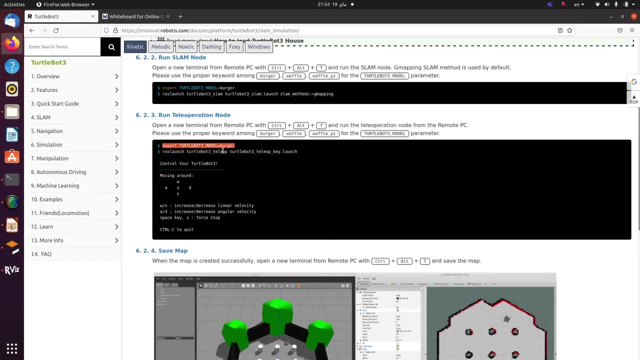 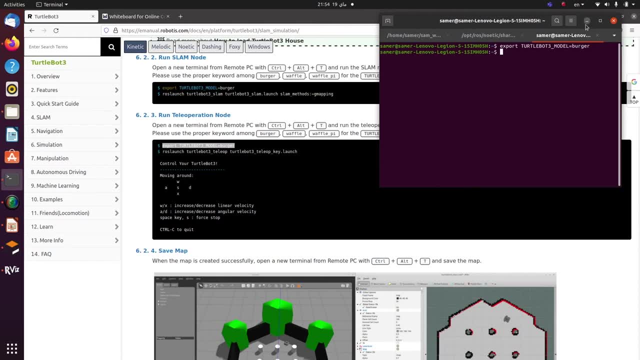 Right, I'm going to copy the robot model, I'm going to paste it here And then I'm going to cross launch my teleoperation node. So now I could, you know, navigate through the environment. All right, So my teleoperation node is now active. 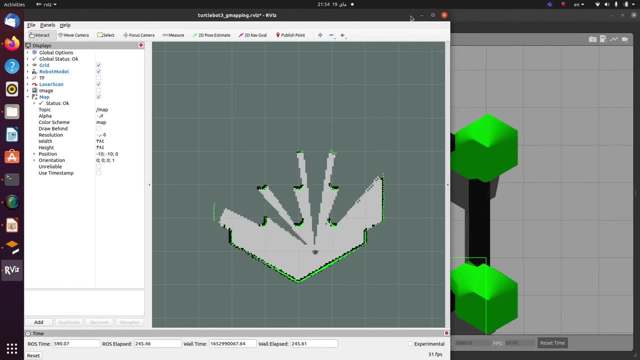 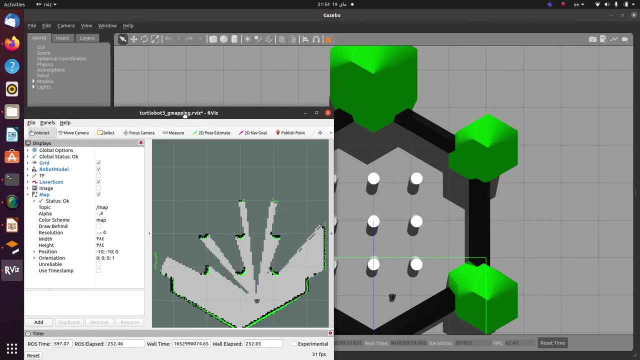 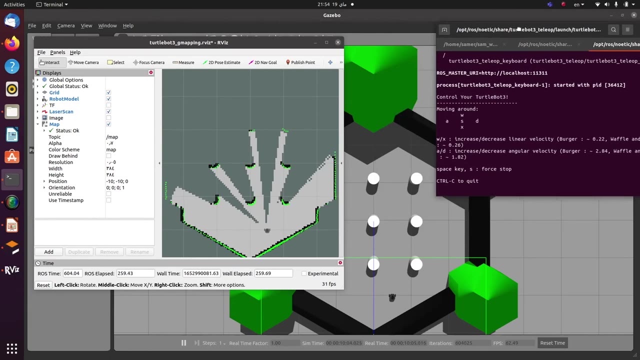 So we're going to visualize Gazebo and our vis. So let's just, You know, like, minimize that a little bit so that we can have a view of everything. And one thing is: I cannot teleoperate without having the teleoperate terminal like open. 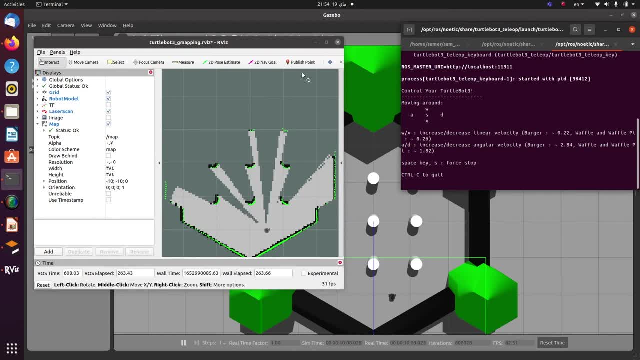 So I need to keep all- Sorry, I need to keep all these you know tabs open, So let's move forward. for example, So I'm going to give some forward linear velocity by clicking W, So I'm clicking W. 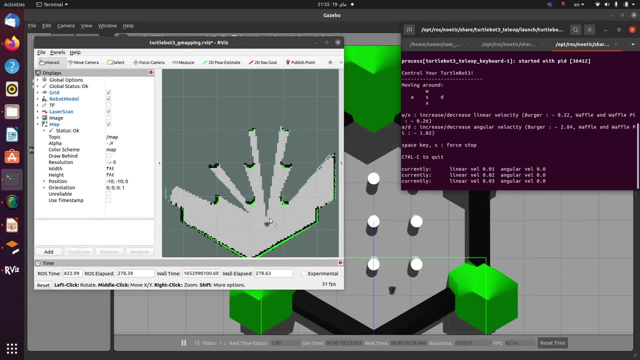 You could notice here that you know the map is starting to look more, you know, complete. We are gathering new observations And these new observations help me, like, construct the map. So the locations that weren't obvious or were vague are now close to me. 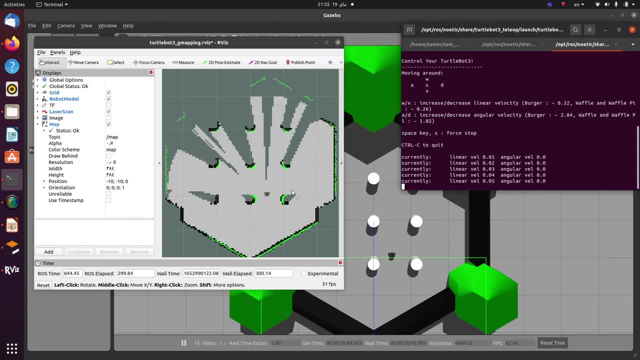 And now I can get new observations. And I begin to, you know, overlap these new observations with old ones, And I'm beginning to, you know, construct a better map And at the same time I'm localizing my robot. 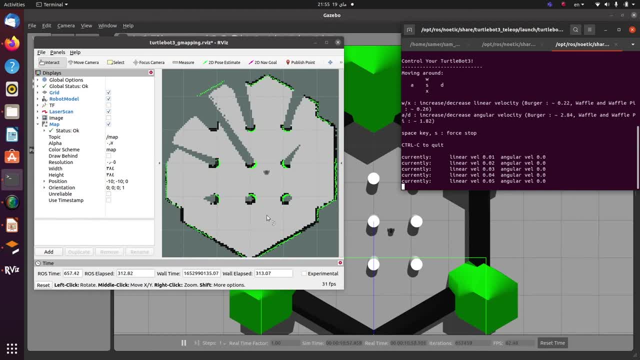 All right, Because I didn't have any information about the location except the very first location that I had here And I assumed it's the initial location. So I'm referring all the upcoming locations to this- you know starting location And I'm trying to figure out some, you know, some intuition behind my current position. 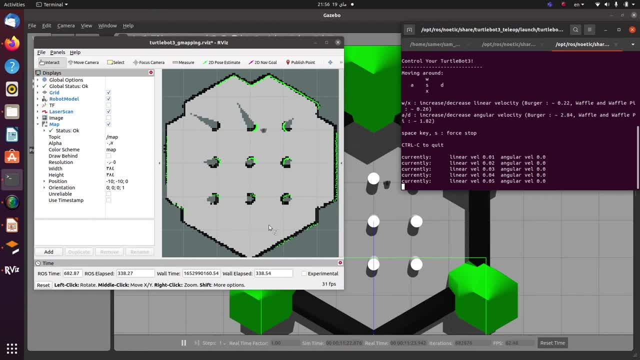 Based on all this information, Based on all this information that I'm gathering over the simulation time span. All right, So you can see that I so far I have a pretty good you know- understanding of my map. So I mapped most of my environment. 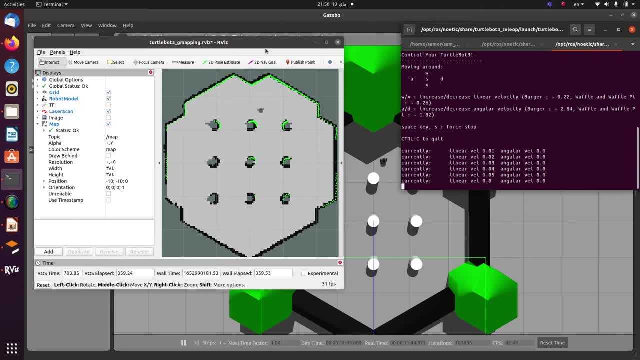 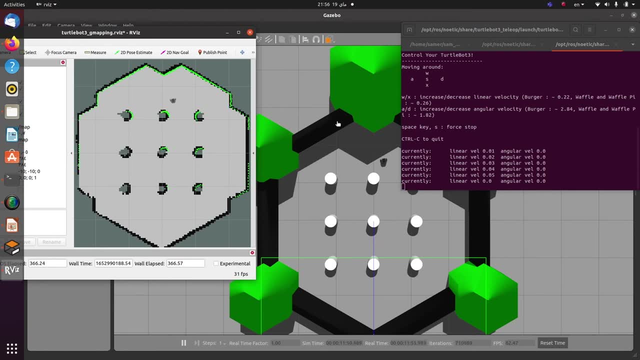 All right, But only the part of the environment that is located within the turtle bot house or world, Because you can find that this is a closed world. That means my robot is like in a closed environment, So I cannot map what lies beneath these walls because this is a closed place. 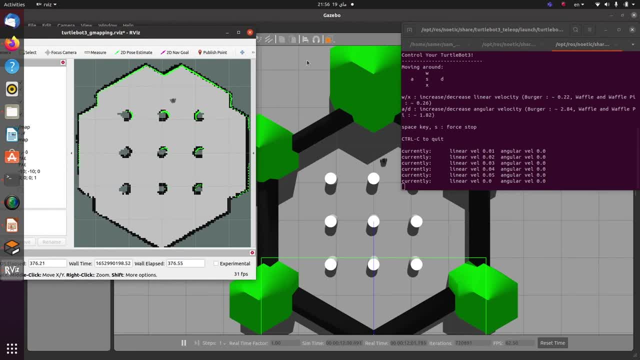 It's like a castle, All right, So I can't possibly map the environment that you know or anything that lies beyond these walls. All right, Because my LIDAR cannot access anything And even if I get close, I'll just collide with one of the walls. 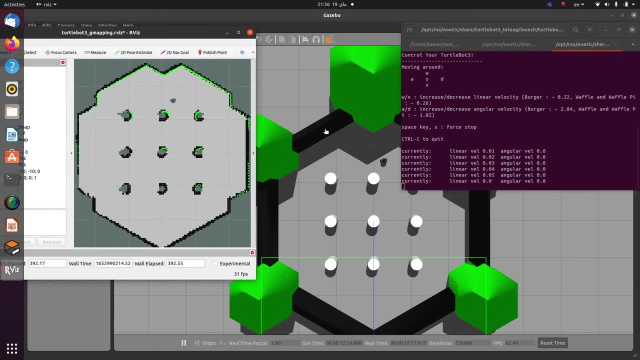 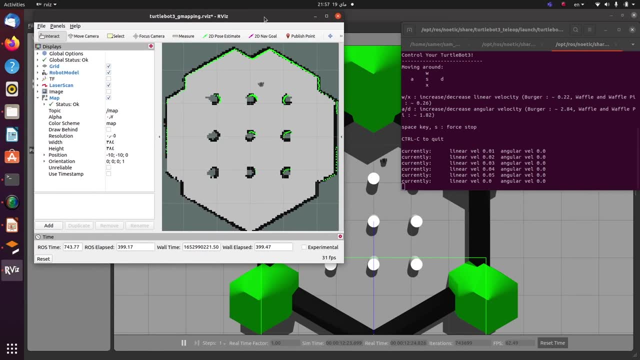 So my biggest achievement here, The only thing that I could achieve- is this: The only thing that I could achieve is like having a map of this closed environment, And this is pretty cool because mobile robots usually operate within closed boundaries or some warehouse or some closed environment. 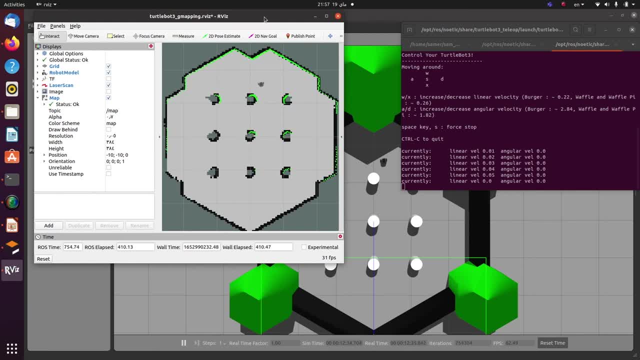 Or, as we say, mobile robots tend to operate indoors. Some robots operate outdoors, But these robots deal with- you know- more complex aspects like dynamic environments. So in this environment you get everything. you know everything. here, Every object is static. 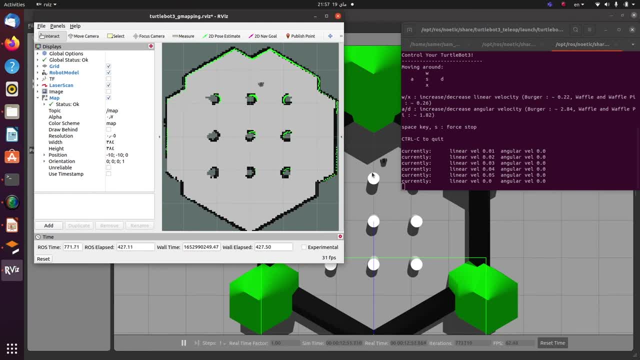 It's not moving. But once you have moving objects, then that would like confuse the algorithm, because the algorithm assumes that the robot is the only thing that's moving. All right, So once something moved, it will you know. it may distort the localization data because, like I was supposed to measure the relative distance between me and the object. 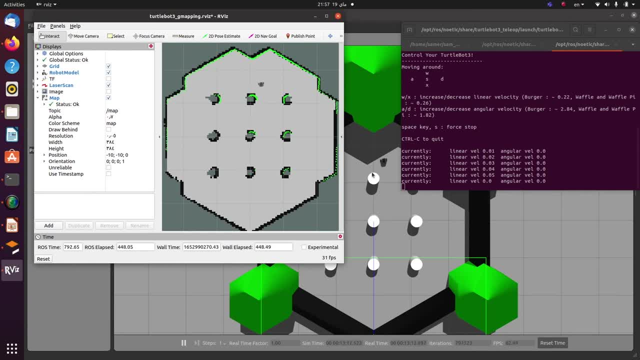 So the object is supposed to be static and moving, But let's just assume that the object is moving as well. So if the object is moving, as you know, with the same velocity as me, then I would think that I'm not moving at all. 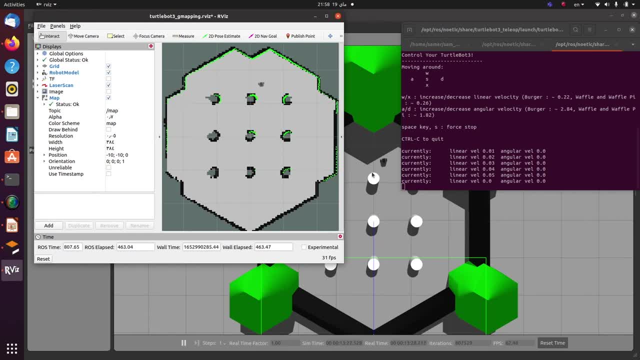 All right, Because the relative velocity is zero. So I cannot, you know, figure out whether I'm moving or the object is moving, or both not moving. So everything has to remain static. So that's why, in the standard situation, we operate indoors. 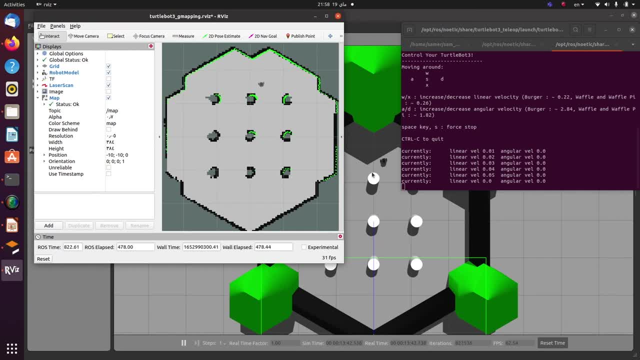 But when you operate outdoors and the presence of dynamic objects like people and cars and stuff like that, the problem tends to be much more complex And this requires a lot of research work in order to work in such environments. So this is a pretty advanced level. 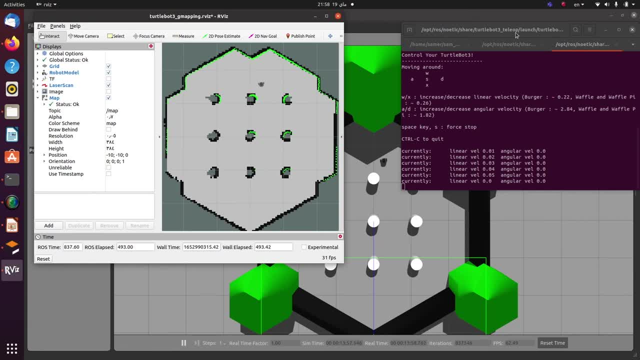 We're not going to go through that, All right. So I can notice that some parts are still distorted. For example, this part seems, like you know, not completely mapped, Because when something is completely mapped or when some object is completely mapped, 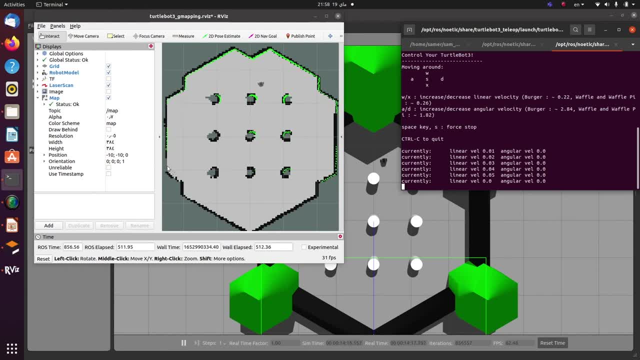 then it's going to have like some sort of distortion, Some solid boundaries, some solid black boundaries, So this, for example: I think this one is open, So I don't really know if there's a wall here or is it open. 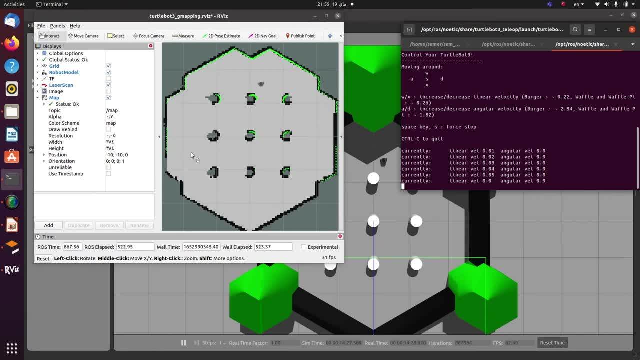 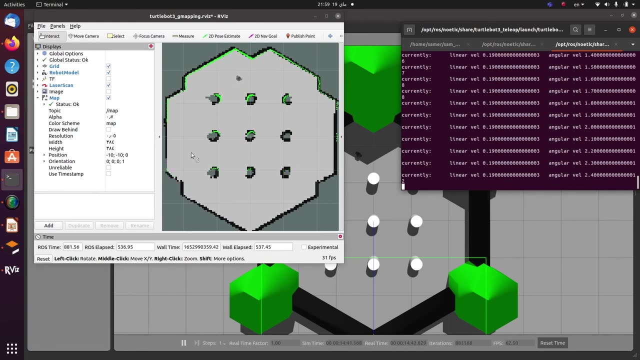 So I need to, like, rotate a little bit and just continue navigating my environment. So I'm going to rotate a little bit, All right, Yeah, Then I'm going to stop, Then I'm going to move forward and rotate a little bit. just to you know, I need to change my trajectory. 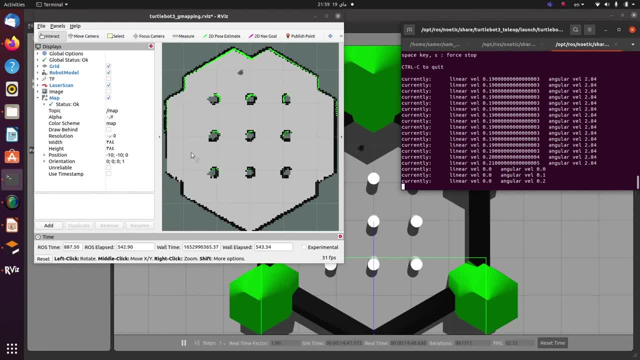 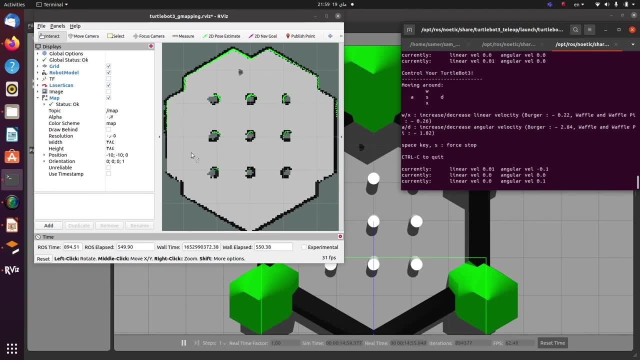 All right. So I started rotating like crazy. So I need to adjust myself. Now I move forward. Stop again. Then I move forward here A little bit faster. All right, Stop. So we can notice that each of these cones in the middle 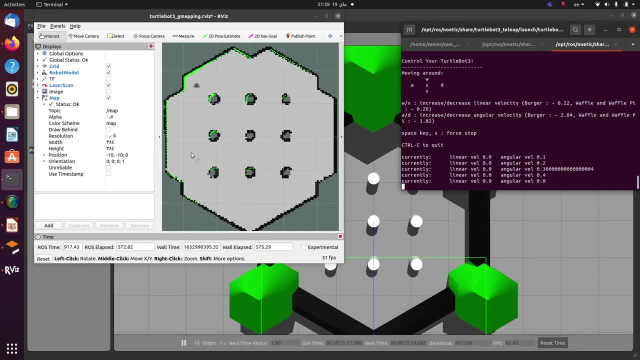 are now, like, totally encompassed by black dots, except this one here and this one, But I'll get to them later, So I'll move forward now. As you can see, these open areas are now, you know, encompassed with black dots. 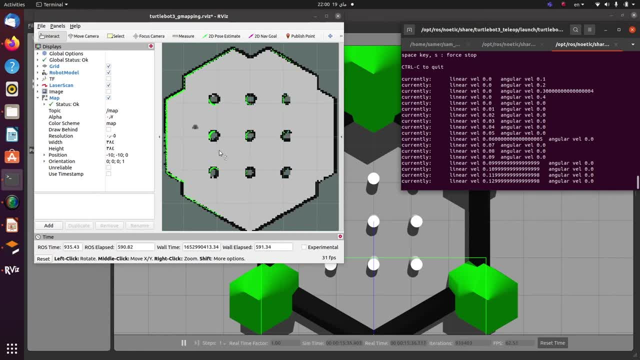 So I'm going to have a black dot here. So I think now it's closed, And the same thing goes for that area here which was open. Then I'm going to stop in order not to hit the wall, Then I'm going to rotate a little bit. 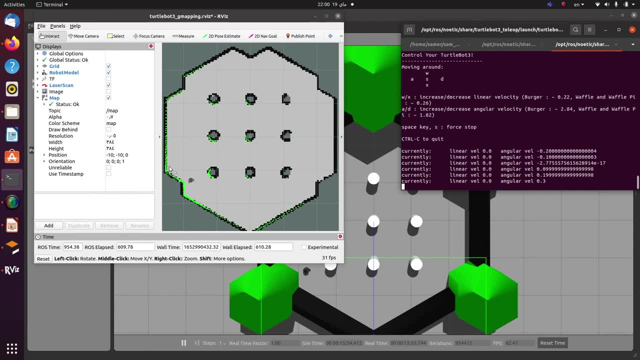 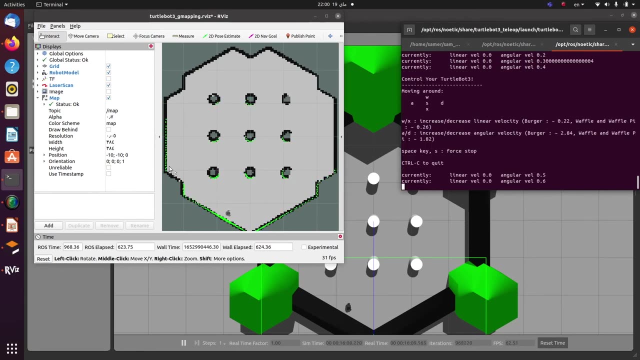 Now in the other direction. So, yeah, I'm going to move forward now A little bit faster. I'm going to stop, I'm going to rotate a little bit in this direction And I'm going to move forward again. All right, 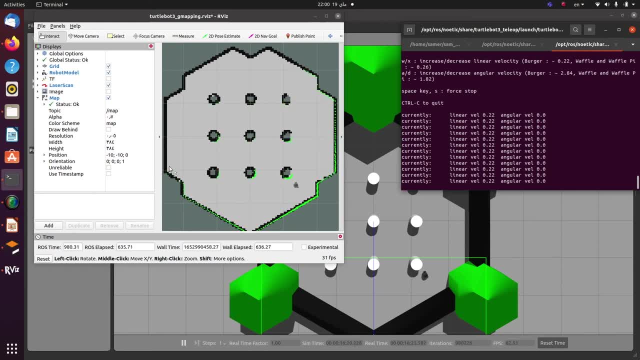 So I need to close up these cones here, These white cones. Then I'm going to rotate a little bit So I'm gaining new observations. All right, So I'm going to move forward again. So yeah, now I need to just close these two cones here. 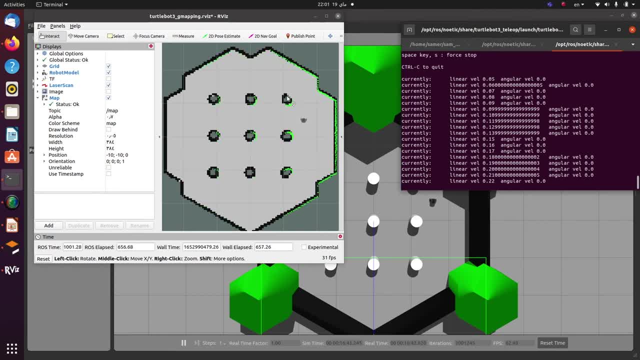 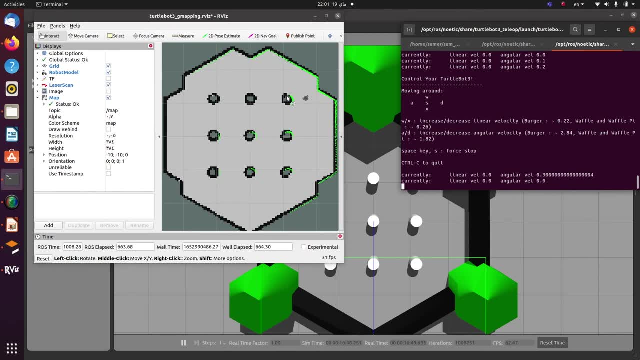 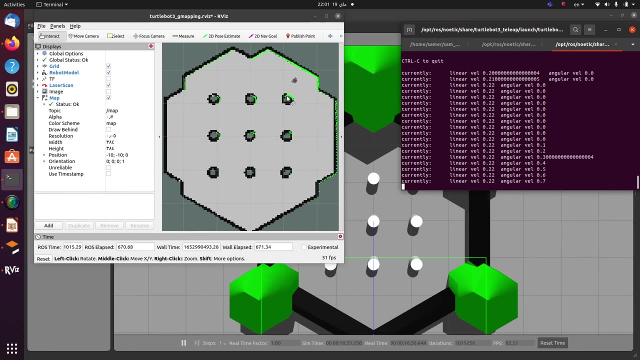 And I think the map would be ready. I think I'll be done with the entire map. I'm going to finish up this cone here. So, yeah, I think the map is complete. now if I look, Yeah, I think the aspects of the map are complete, or you know. 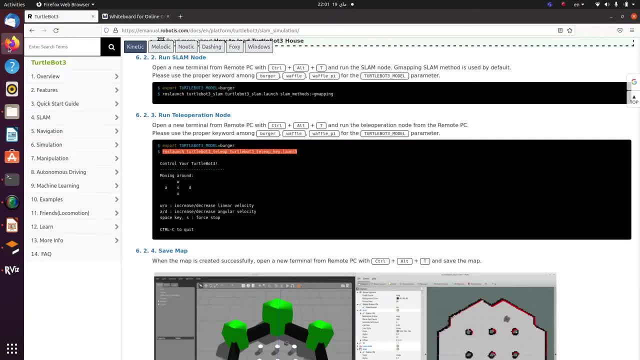 Yeah, I think that's enough so far. All right. So let's get to the next step, after mapping my environment through teleoperation node- And, by the way, I'm not just mapping my environment here, because I'm using a G mapping algorithm- 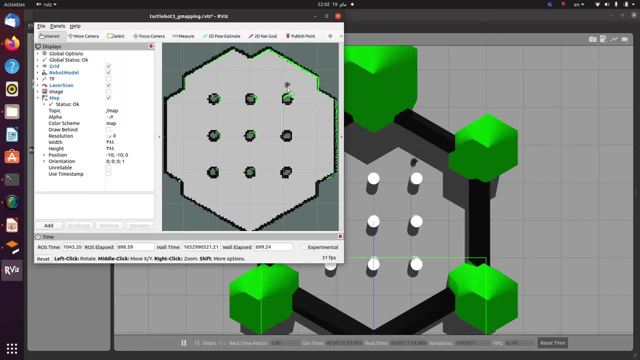 So I'm both mapping and localizing my robot, But the localization part is not, you know, visualized here. Only the mapping part is visualized. But once you have a map like this, you can always make sure that there is some localization node running somewhere. 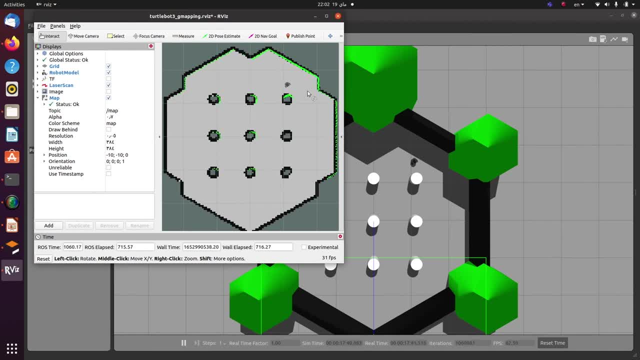 Because I cannot construct a map, And if I'm, you know, executing individual mapping, then I must have the location of the robot somewhere from a GPS sensor or something. So you can, you know, know that, rest assured, there is some localization node running right. 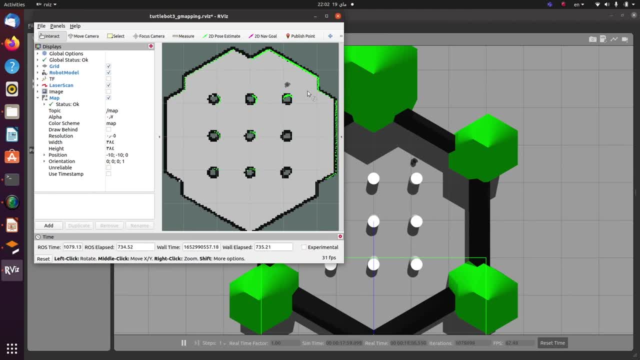 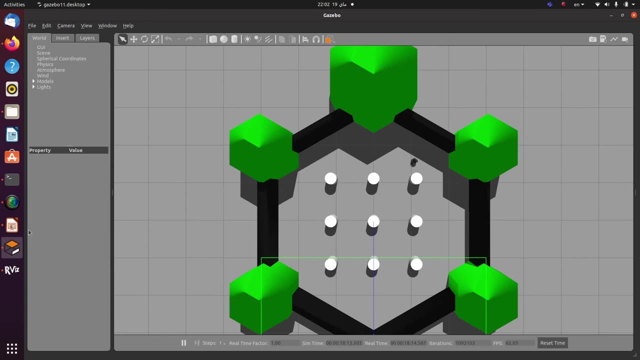 Whether you're doing SLAM, which is simultaneous localization and mapping, or doing some individual mapping and you have the localization data coming directly from a sensor, All right. And if you're doing G mapping, which is a SLAM algorithm, we know that we're both localizing and mapping at the same time. 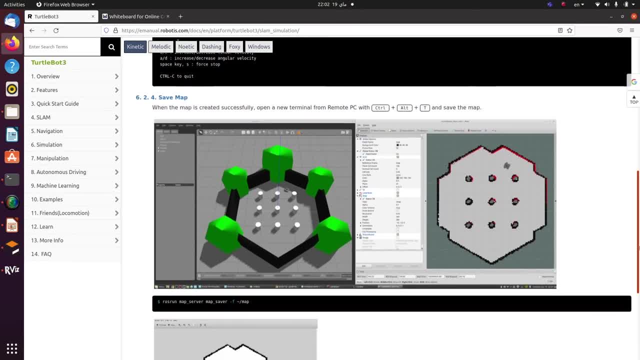 So let's get back here Now. I need to save my map- All right, The map was created successfully. I need to open up a new terminal- All right- And save the map by using the map server. So the map server is like a node. 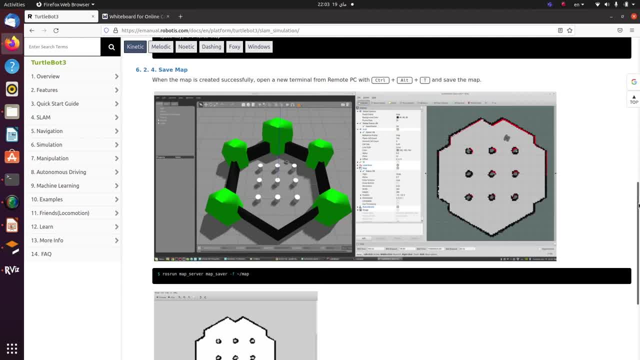 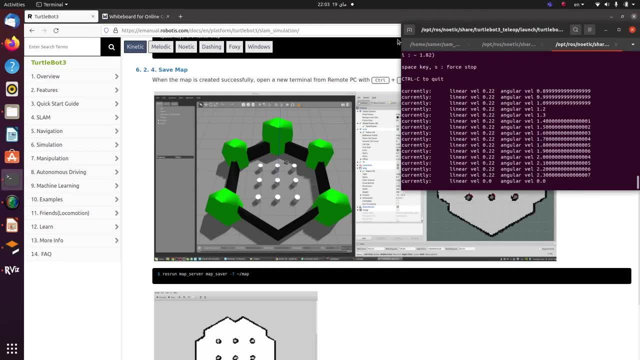 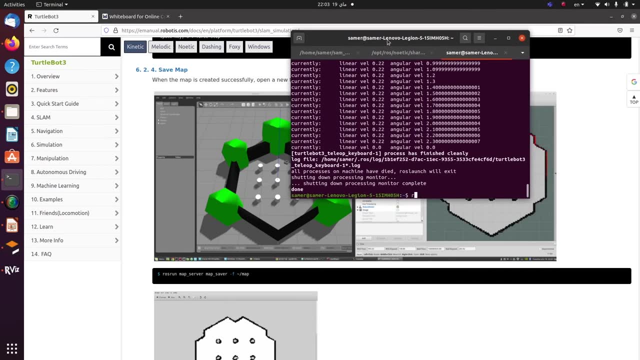 All right, Which gives you some, you know, mapping utilities, like saving the current map that was developed so far. So there's a topic called map here somewhere. If you get to you know, let's just close the teleoperate node and let's you know ROS topic, echo or ROS topic list the nodes that are currently the topics that are currently running. 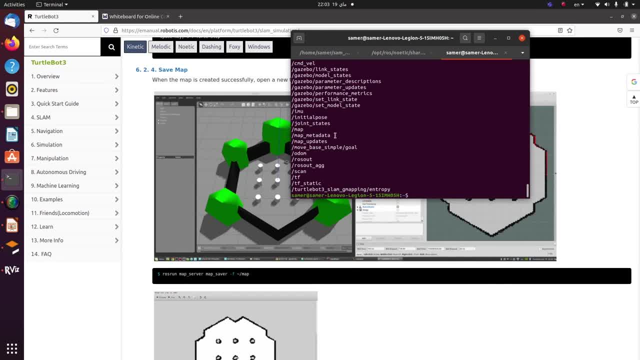 So you'll find a map here and a map metadata and map updates. So there are multiple map topics here. You know these multiple map topics include information About the map that was constructed so far. If I, for example, echoed this map topic, 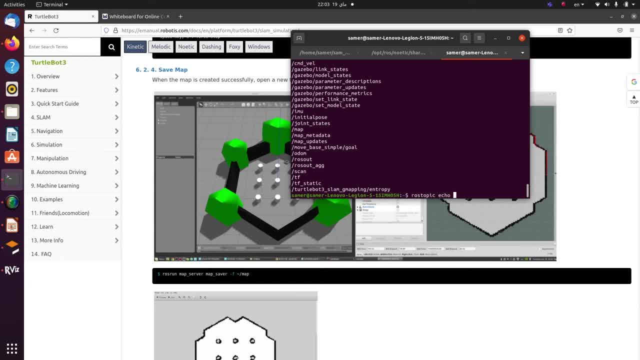 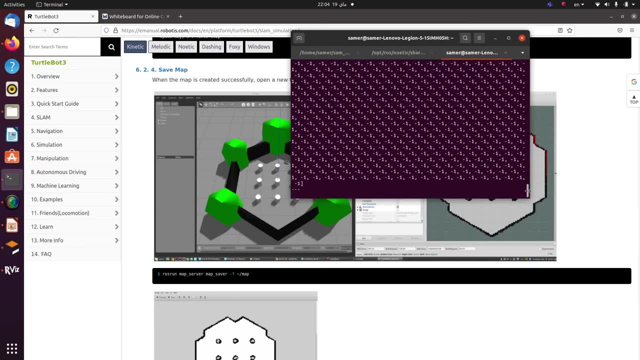 So I'm going to type ROS topic echo map. So you'll find that there is a matrix here And this matrix is quite huge. actually I cannot, you know like, determine what's going on. actually You'll find a number of zeros and negative ones, and maybe ones. 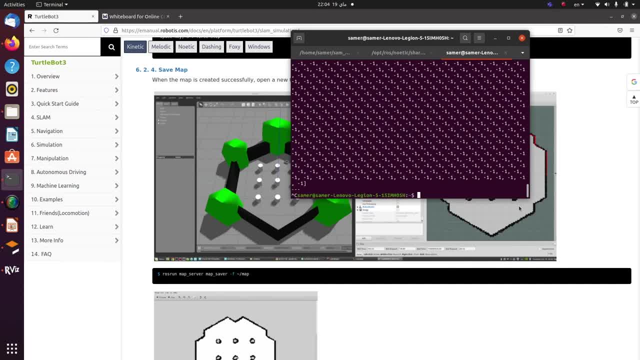 So each of these, you know each of these numbers represent, you know the number of nodes that are currently running, And each of these numbers represent a certain fact. For example, negative one means this is a pixel in my map, And by a pixel I mean like a small square within my map or a small digital portion of my map. 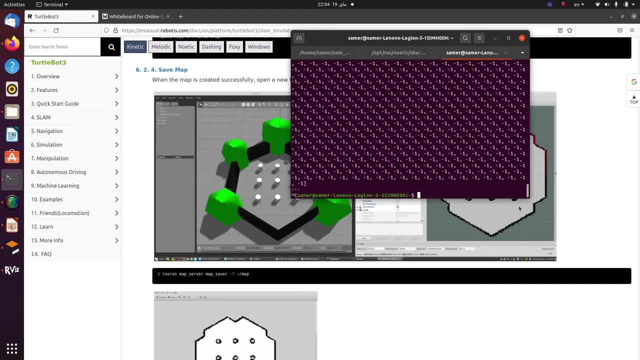 If you're familiar with images, you'll know that each image is made up of digital pixels that make up the entire image. So the same thing goes for the map here And the negative one. values represent The values of the pixels, which are unknown to me. 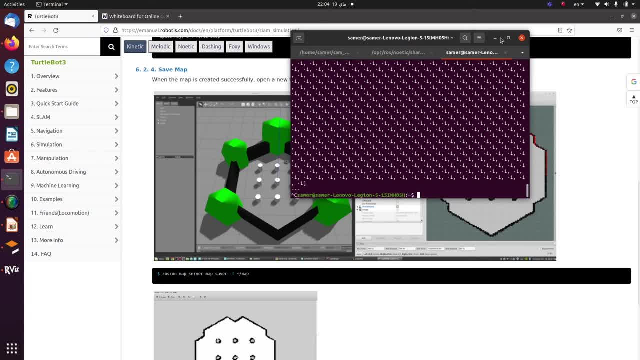 I don't know if something lies there or not, And this probably represents the areas that are outside these walls, The areas that I could not map All right, Which constitutes a very large portion of my environment, Because the closed portion here is quite small relative to the rest of the environment. 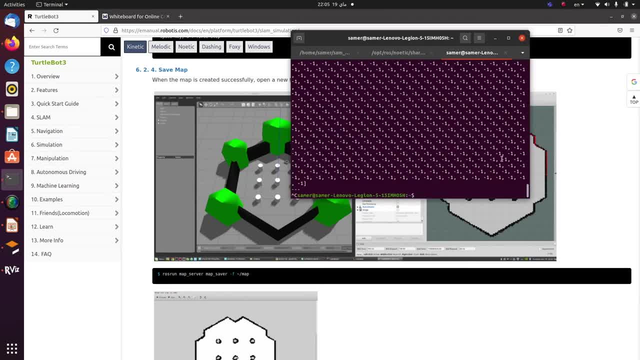 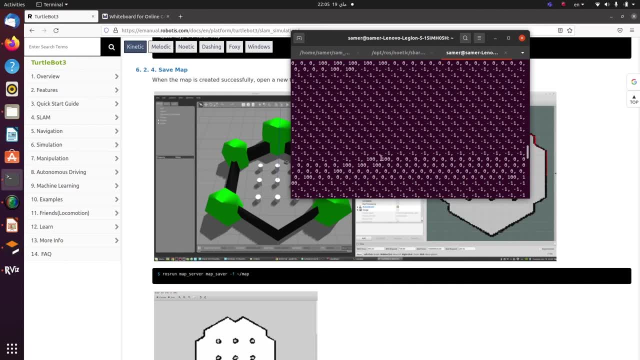 So you'll find that most of your matrix is made up of negative ones, And then you'll find zeros and ones, or zeros and hundreds. here It's not zeros and ones, Zeros and hundreds. So I believe. as far as I remember, I think zero means an empty pixel. 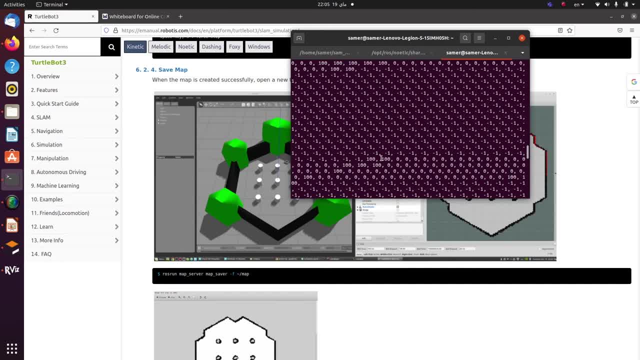 Which means there are no obstacles there, And hundred means that I'm quite certain that there is an obstacle there. So this is a percentage that represents your. you know how certain you are that there's an obstacle in this particular location. So hundred means I'm 100% sure that there's something there. 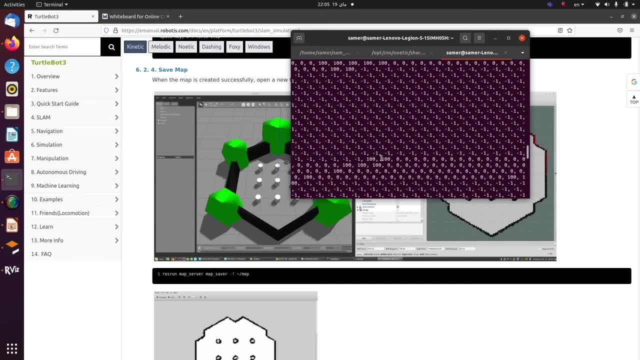 And zero means I'm 100% sure that there's nothing there. So my belief in the presence of an obstacle in this particular location is zero, And while 100 means that my belief in the presence of a particular object in this particular location or particular pixel is 100%, 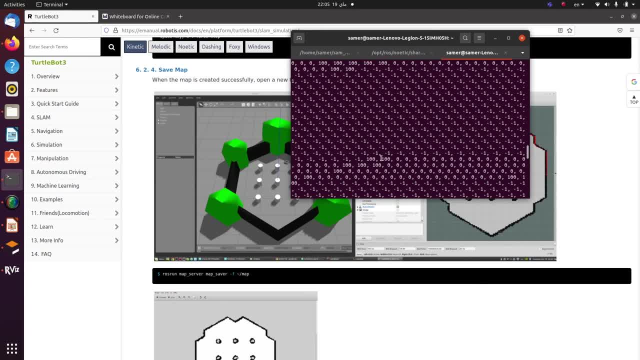 So if you get 70%, this means that there is. you know, you're more likely to believe that there's something there, Right? And if you got like 30% or 20%, which is below 50%, then you're going to use like approximation methods. 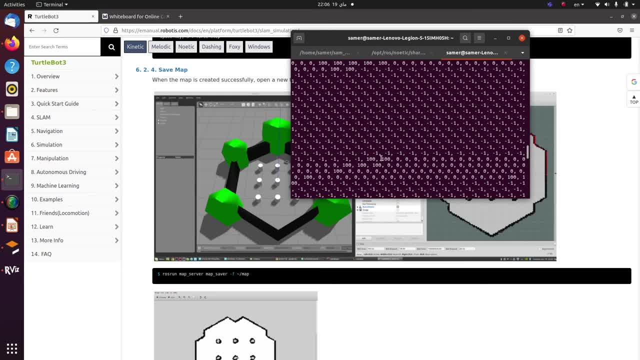 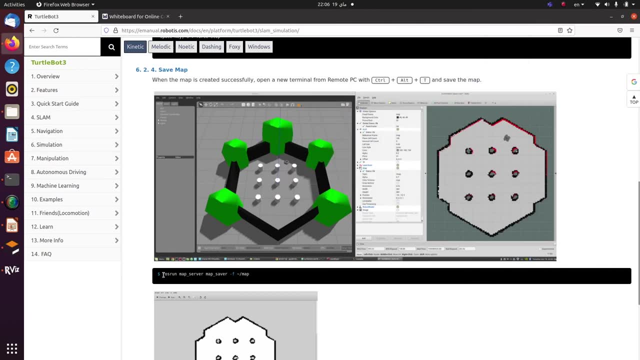 And you know, believe that most likely there's nothing there, But I'm not quite sure. But since LiDAR readings are very accurate, you'll either. you'll probably either get 100 or zero. All right, So we now need to save the map. 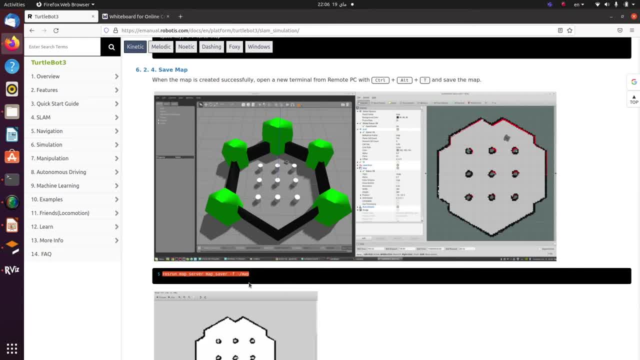 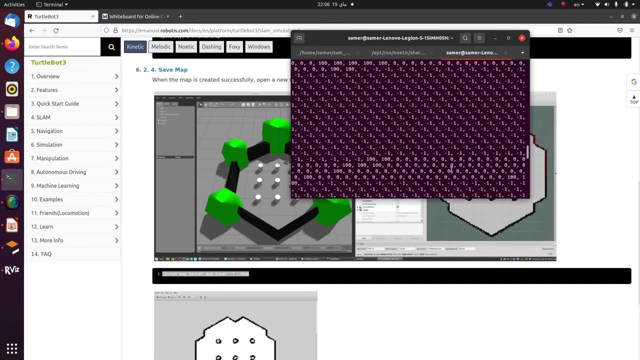 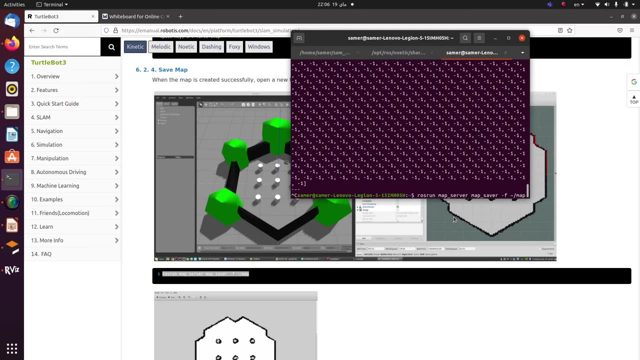 Right Using the map server. So we've got a node here- This is the map server package- And we get a node called the map saver Which saves our map, And we're going to run that Right And I really can't remember where the map is saved. 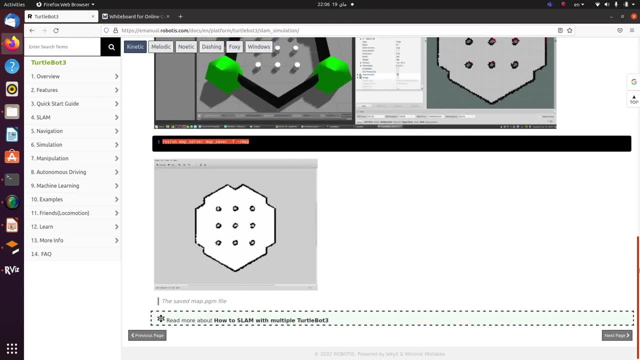 I think it's saved in the home directory by default, And it's saved in the form of something called a PGM file, Which is sort of, you know, resembles a PNG extension or a GPG extension for images, Right? So it's a special type of file designed specifically for maps. 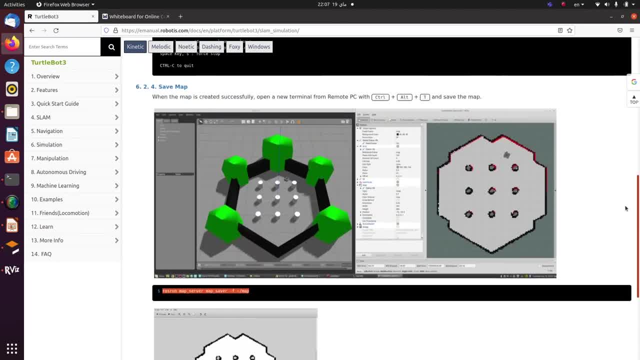 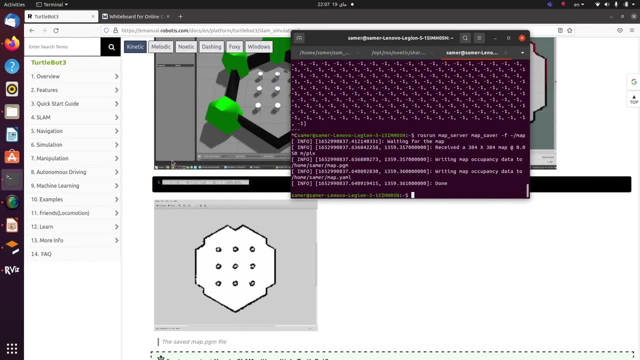 And I think it's saved in the home directory by default. All right, Let's just check it out. Let's run it. All right, So it's done. Yeah, Here. It said that it showed the map occupancy data, And by occupancy I mean it's a map that you know indicates whether each of its pixels is occupied or not. 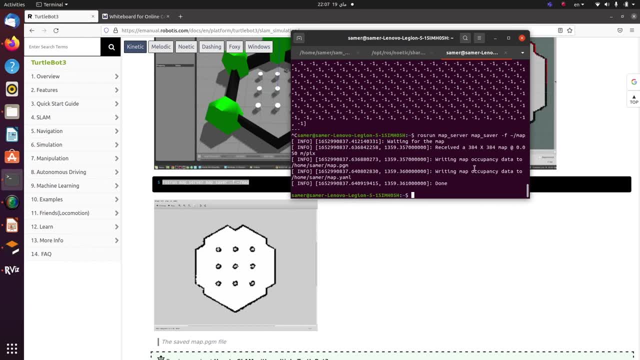 So this is why it's called. sometimes a map is called an occupancy grid Right And it's saved to home somewhere: mapyml. So yeah, So a map is saved in the form of an M file and a PGM file. 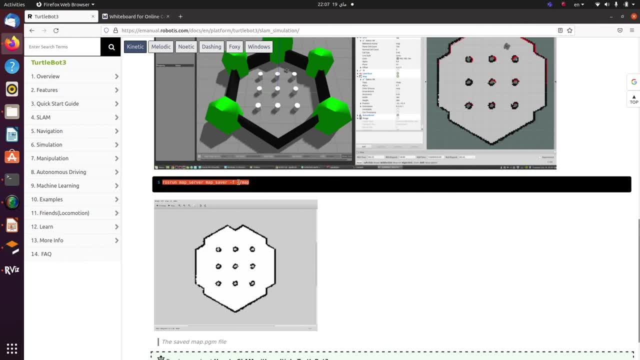 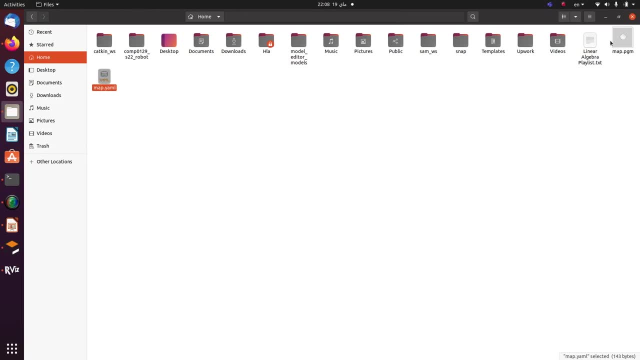 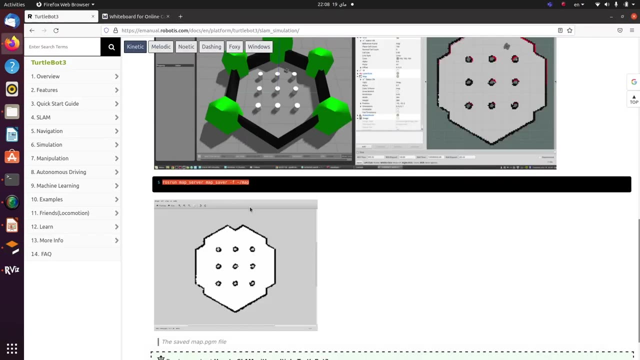 Both extensions come out of this map server. So if I head to my home here I'll find, yeah, I got mapyml and mappgm Right. You'll find them here in my home directory, Because this command line, Because this command by default saves my map in the home directory. 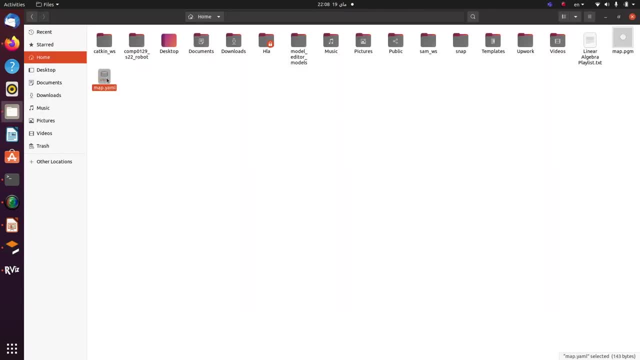 And let's try to open up one of these files. For example, let's open the CM file here. So yeah, It's saved in the form of an image having the extension PGM. So this is the location of the image. 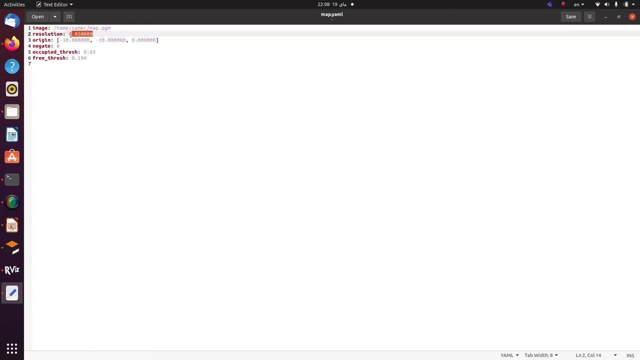 And this is the resolution, And by resolution or resolution of the map, I mean that each pixel has, you know, is in the form of a square that has like 5 centimeters side length, Because 0.05 is a meter. 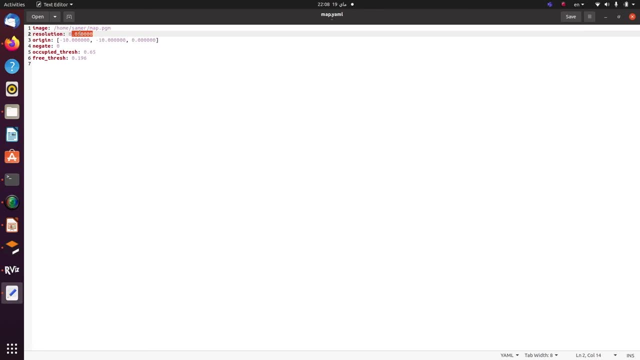 So you convert that to centimeters And it's like 5 centimeters. So you got pixels, square pixels, each of them having 5 centimeters. So you digitize the entire environment into you know a number of these pixels. 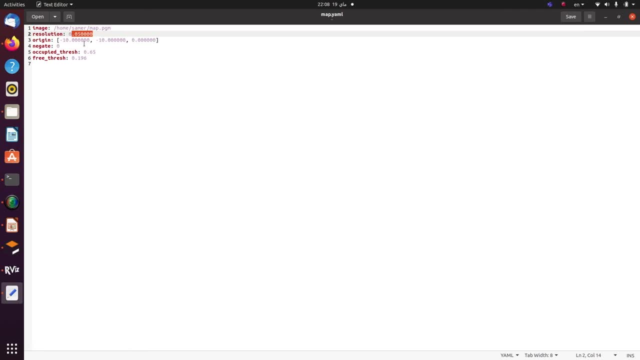 And you've got the origin. So the origin of the map is negative 10, negative 10, and 0. That means that your X coordinate of the origin of this map is negative 10. And in the X direction and negative 10 in the Y direction. 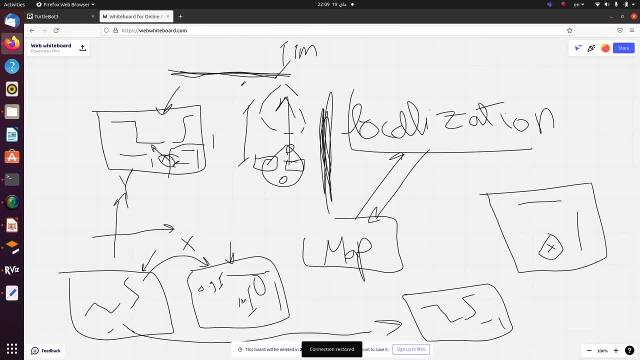 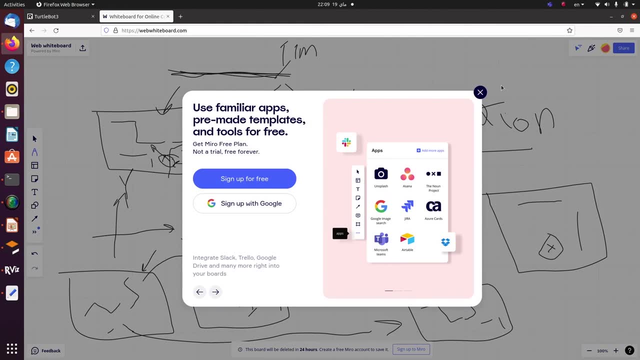 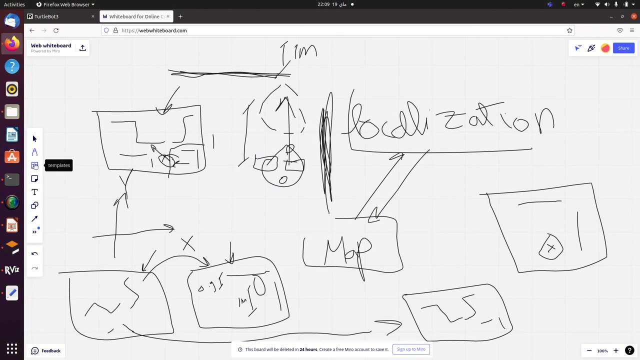 What this means is, for example, if you open up a whiteboard here, Let's just try to. you know. I think there is right. I think I'm not allowed to use, I'm not allowed to use, an eraser. 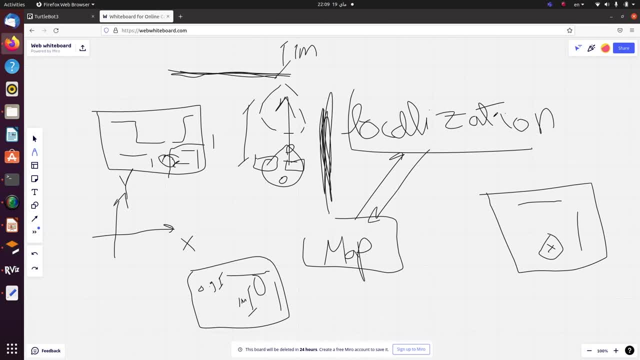 All right, So I'm going to just delete some of the drawings I had here. So So, basically what this means: if this is my environment, All right, And usually in Gazebo environments, the origin of Gazebo itself is located somewhere here. 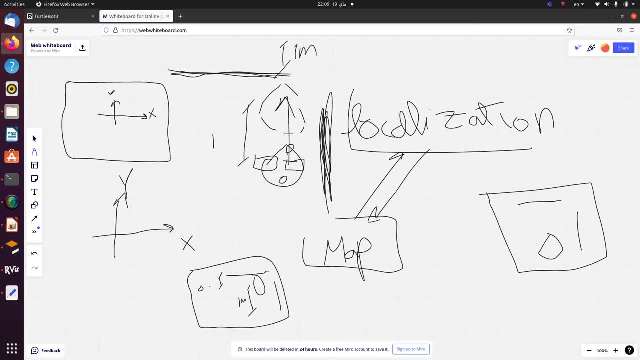 In the middle Right. So this is the X and this is the Y, for example. So the origin of the map itself, or when you're, you know, using the map server, The map server has, you know, a picture format. 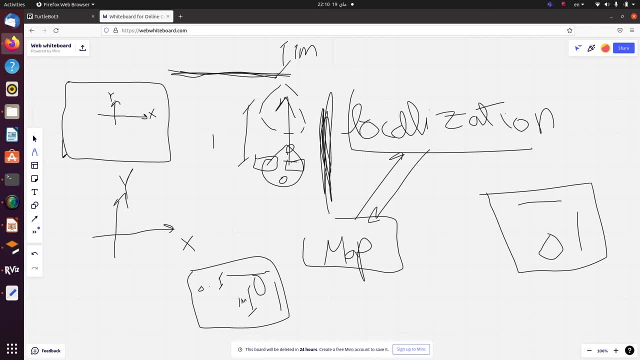 So in picture formats You can see that your origins or the origin of the picture is somewhere here, Right At the beginning or at the end, At one of the edges, Right At one of these vertices, Right. So yeah, that's usually the case for PNG, GPG and PGM and such extensions. 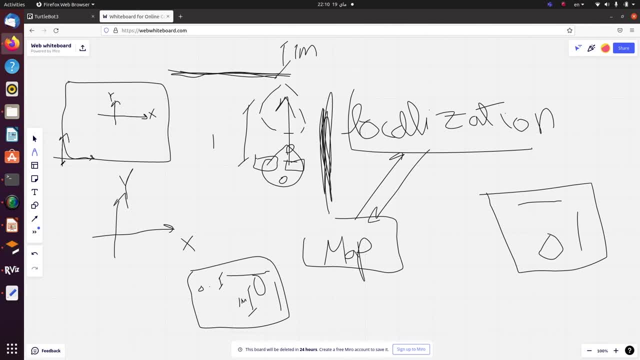 Usually the frame or the origin frame of that image is located somewhere here at one of these vertices, And what basically says is that The origin of the of the image is like negative 10 meters away from the origin of Gazebo, And negative 10 meters away from the origin of Gazebo in both X and Y directions. 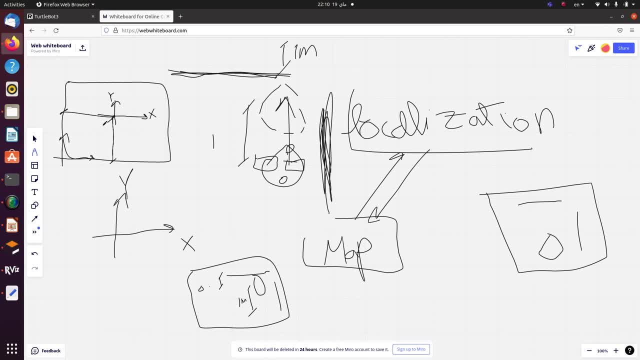 So this is just to you know: offer some sort of transformation between Gazebo's origin frame or fix it frame and the frame of the image itself. Right, And let's get back to the end And I'm fine. I think it was down one. 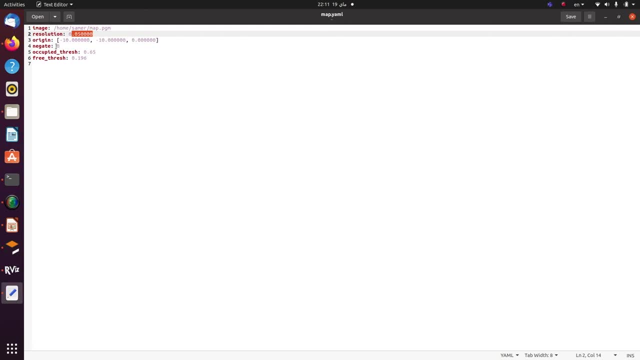 Yeah, Negate. I'm not sure really what negate is, but the occupied threshold. This is the threshold after which you can say that this pixel is occupied. All right, So once your reading exceeds 0.65.. And I believe that 65%, I guess, because it divides the map pixel values by 100 in order to obtain some probability. 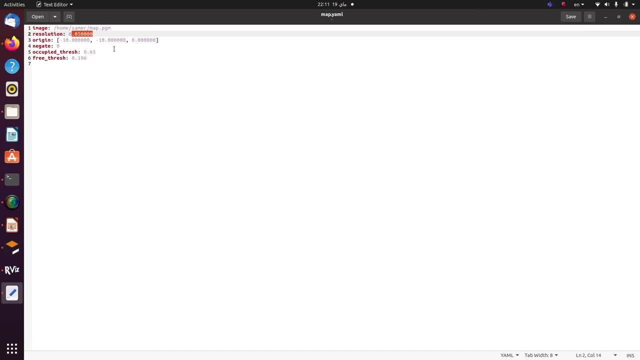 Right, Because probability is between 0 and 1.. So you have to divide 100 by 100 or divide your percentage by 100. So I think 0.65 here. First, the fact that once you see that your pixel is like a pixel value exceeds 65%, then you can consider that this pixel is occupied. 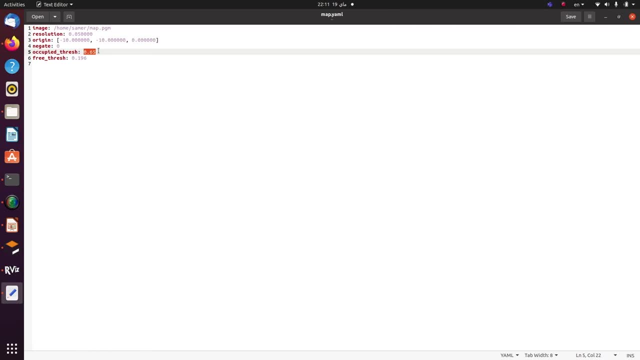 And the free threshold. So once you're less than 0.196, which is almost 19.6%, So you can consider that this pixel is free. All right, I know I said earlier that it's 50%, but that depends on the algorithm itself. 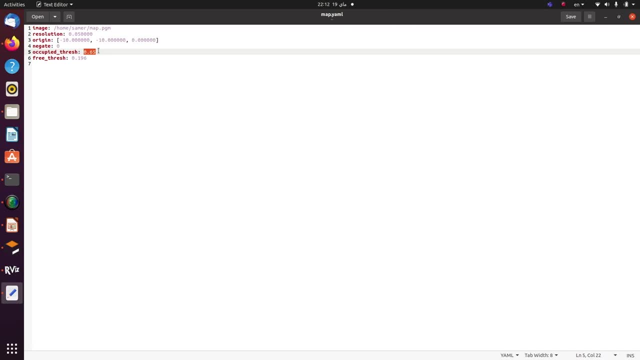 So for the algorithms I write myself, I usually pick the threshold 50%, Right. But here the designer had another opinion, All right, And it differs from one designer to another, So we got to go with that Right. And if you open up the PGM file here, let's open it up. 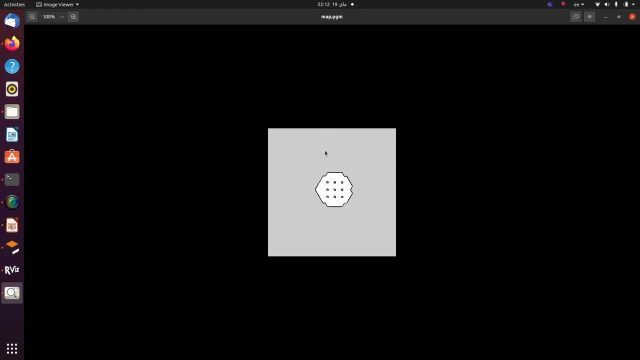 So we can find. it's basically an image file- Where the unknown location has, you know, like a gray value, Because this is, like we say, a gray area, An area that I don't know anything about And where I think the gray area expression refers to something that, yeah, is not quite. I cannot tell whether it's occupied or not. 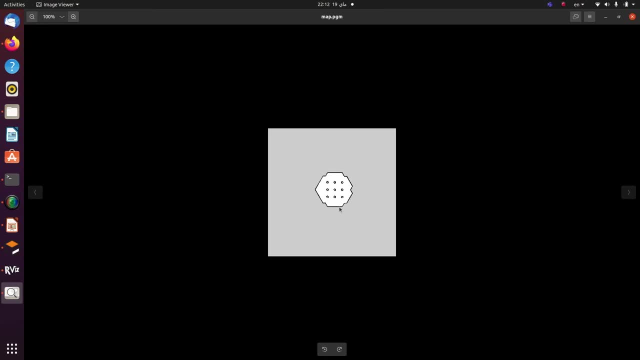 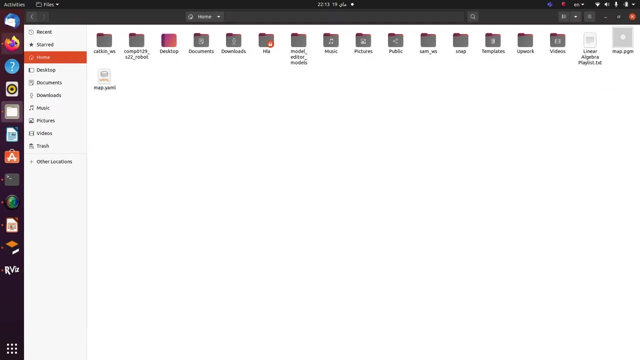 And we've got the black lines which represent occupied pixels, And we've got the white portion here which says that this area is basically occupied, Totally white. that means there are no obstacles within this area, Right? So this is the explanation of what we did so far. 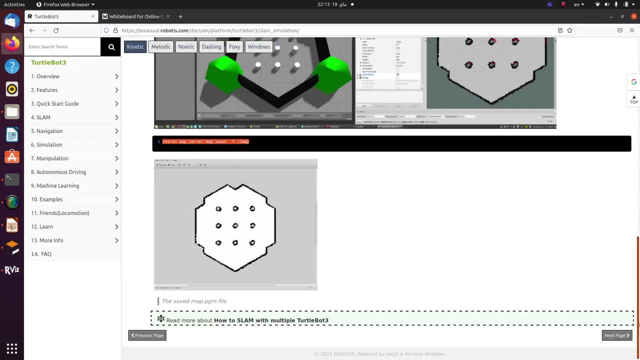 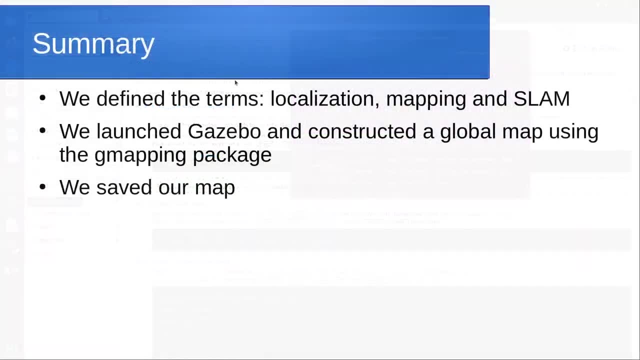 And I think, yeah, we're done. This was the last command here, So yeah, we're done with the implementation part. To sum up what we did so far: we defined the terms localization, mapping and SLAM And determined the- you know the exact intuition behind each of them. 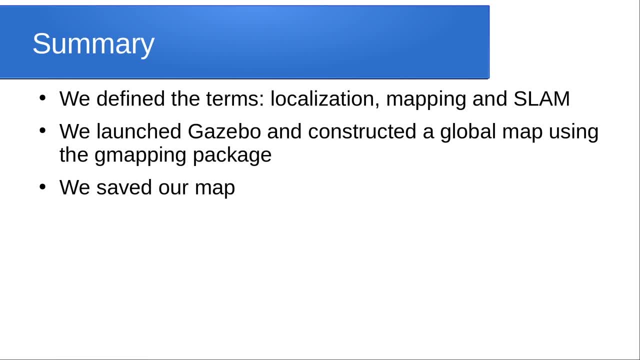 And how localization, mapping and SLAM work. And we launched Gazebo and we constructed a global map using the gmapping package, which is a SLAM package. So we conducted both localization and mapping at the same time And we constructed a global map which kept updating itself through, you know, continuous navigation through the environment.